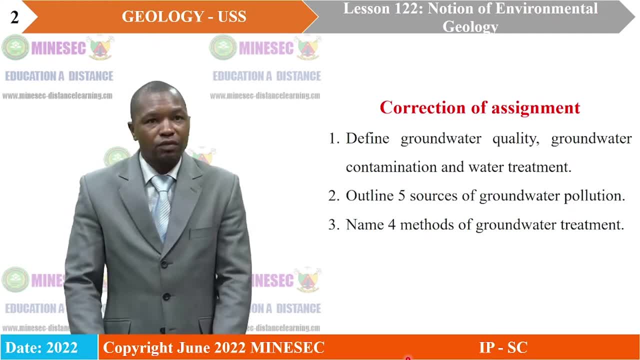 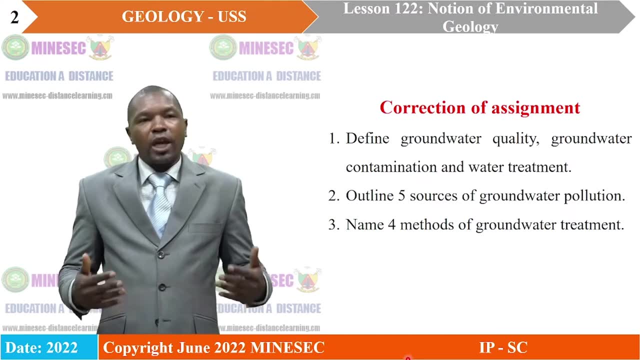 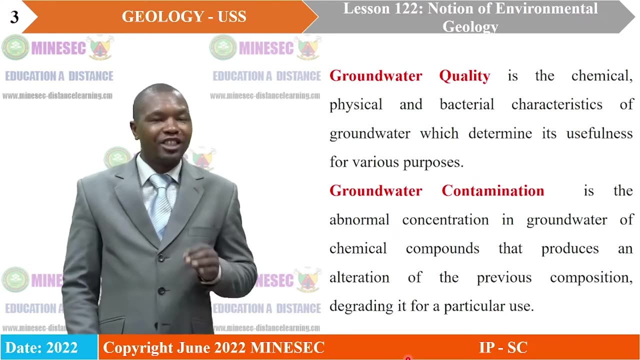 of groundwater treatment. Now, these are AC type questions and we need to, you know, explain a lot of things. So the approach to this question, but one which requires definitions, only has to define groundwater quality, groundwater contamination and water treatment. So groundwater, 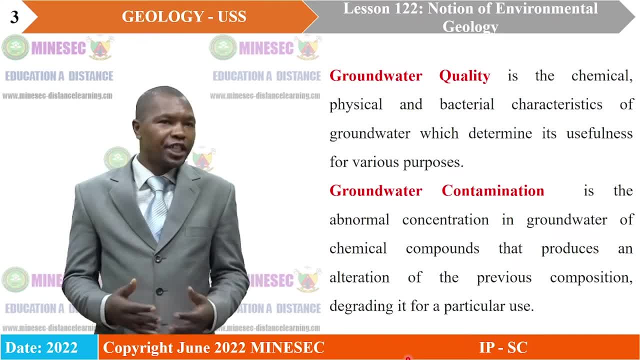 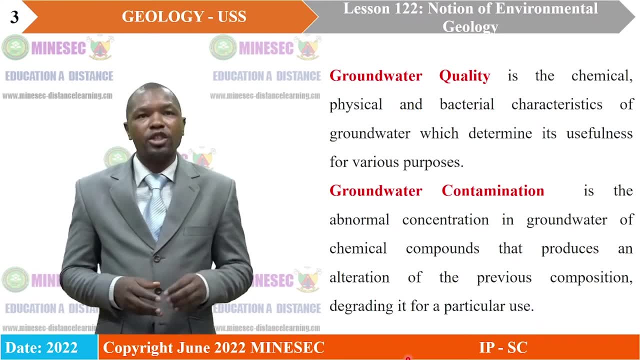 quality is the chemical, Physical and bacterial characteristics of groundwater which determine its usefulness for various purposes. So when we talk quality, we are looking for the chemical, physical and bacterial properties that will determine the use of groundwater for different purposes. Then groundwater is a site of corresponding health or media or services to be used to. 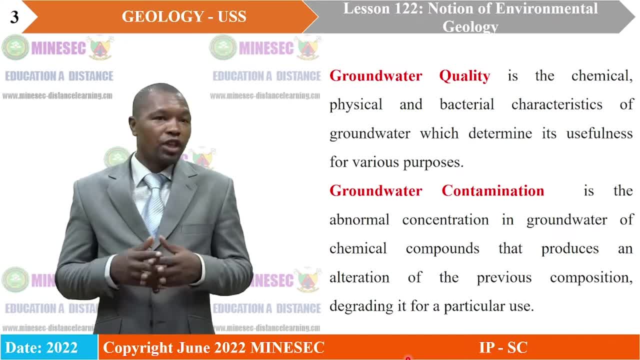 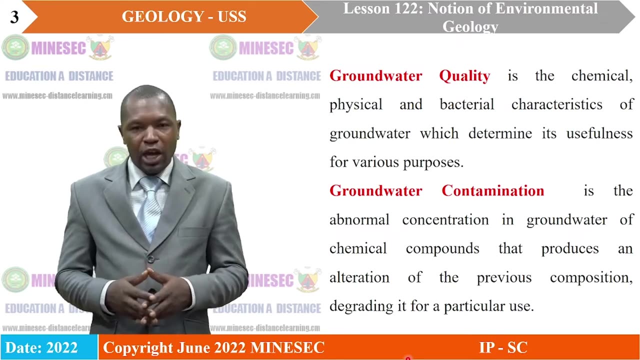 101.3.ai, which is to provide gel, a solution of каждa ille of certifiedным and oral form. analysis contamination is the abnormal concentration in groundwater of chemical compounds that produces an alteration of the previous composition, degrading it for a particular use. In other words, it is the concentration of chemicals or 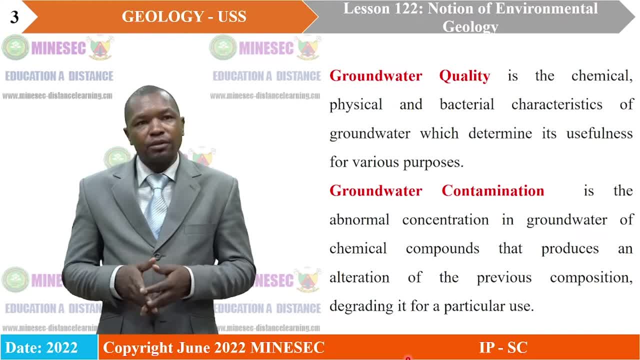 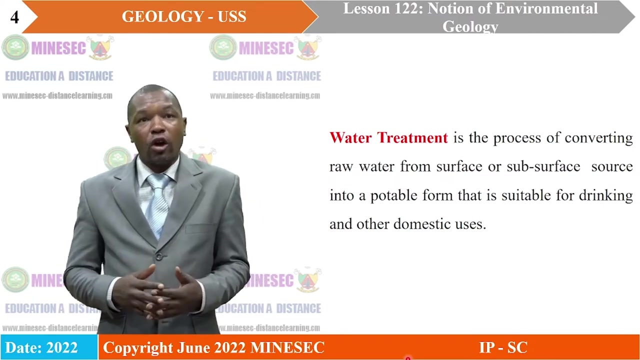 other materials in groundwater in such a way that it makes the composition far from the point of it being used for domestic purpose or for other purposes. So this way groundwater becomes hazardous. Water treatment: It is the process of converting raw water from surface or subsurface. 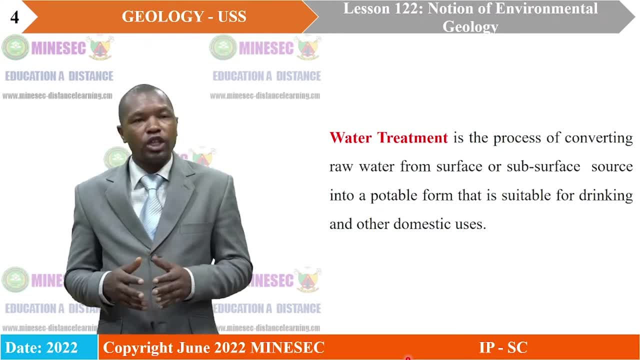 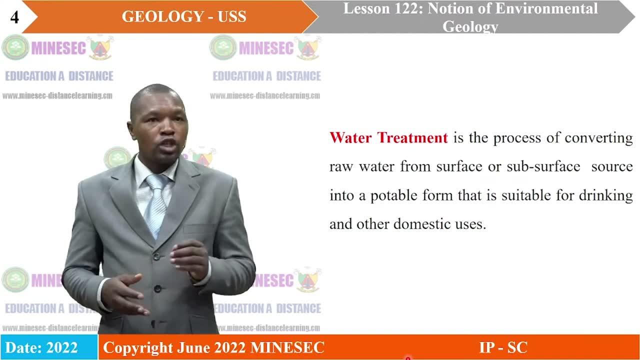 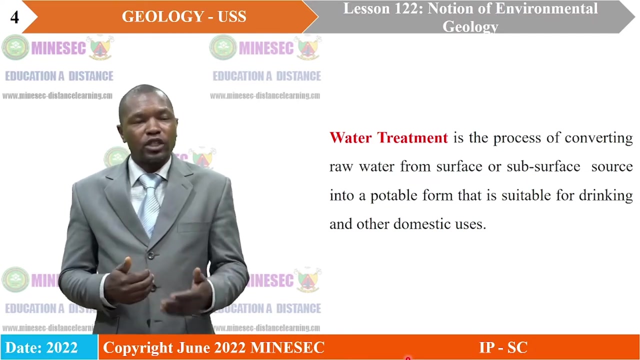 into a potable that is suitable for drinking and other domestic uses. So, in as much as we have water quality, in as much as we have water contamination, we also need to exploit water treatment, because not all of the water that is contaminated is present. So, as long as we have the water two Ahmedmin possesses. 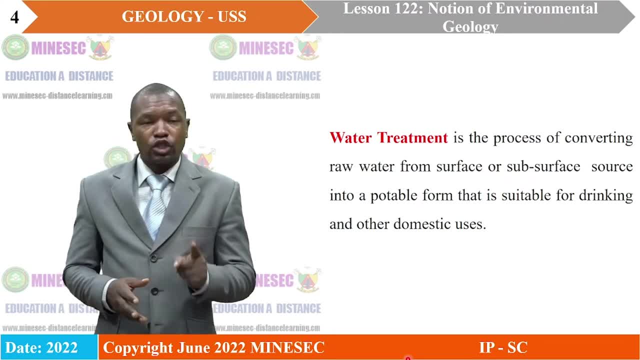 can just go waste. But notes should be taken here, like we emphasized during the lesson, that it is best to prevent groundwater from contamination than to allow it for treatment, because for it to be contaminated is difficult, But once it is contaminated it is. 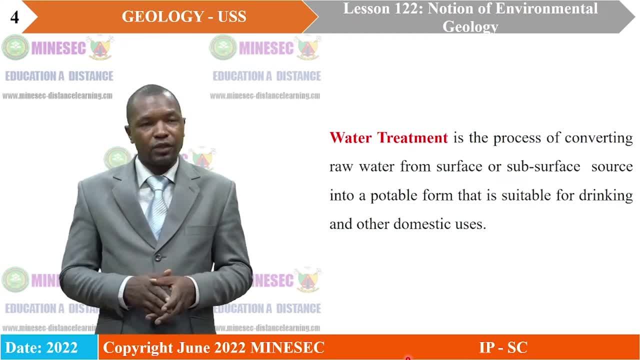 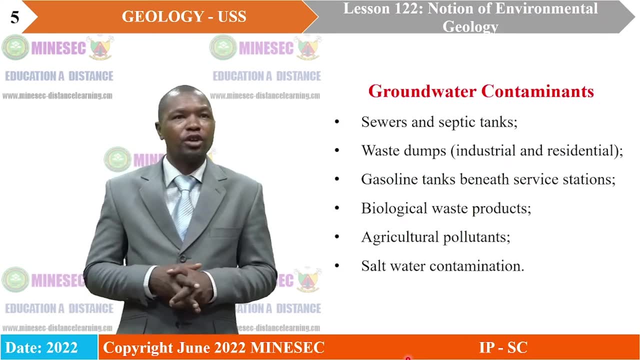 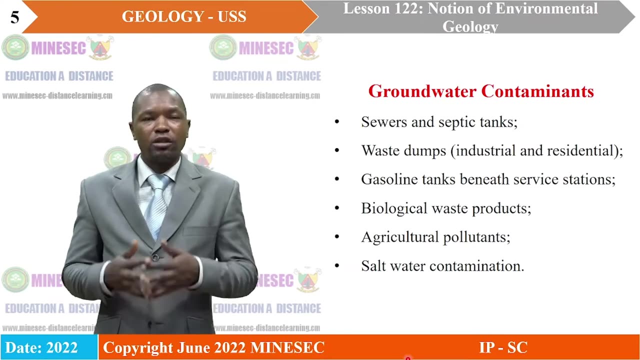 also very difficult to treat it And the treatment is most likely expensive. The second part of the question requires that we should name different sources of groundwater contamination or, better still, name groundwater contaminants. We have seawater and the septic tanks We have. 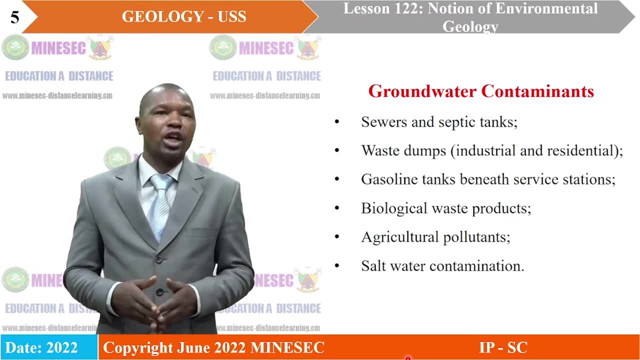 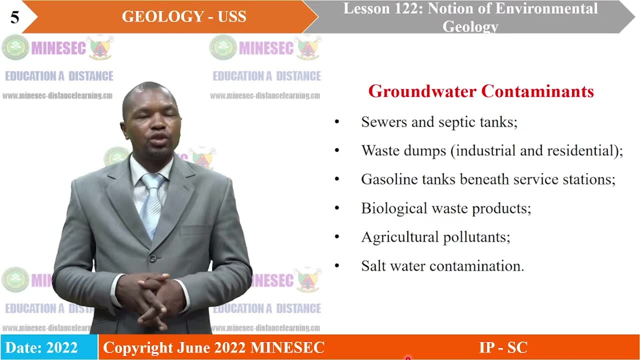 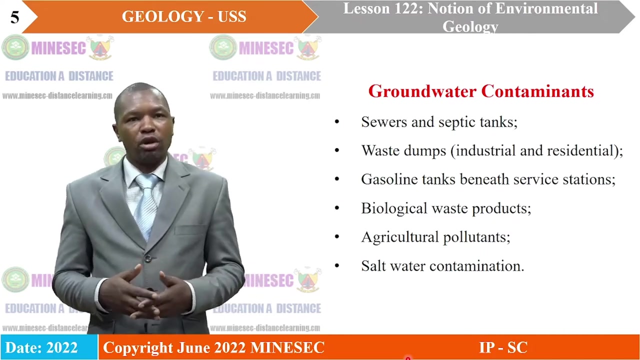 waste dumps, like industrial and residential waste that are dumped in sources where they can leach and get into contact with groundwater. We have gasoline tanks Beneath service stations. they can also leak and they will get to contaminate groundwater. We have biological waste products. 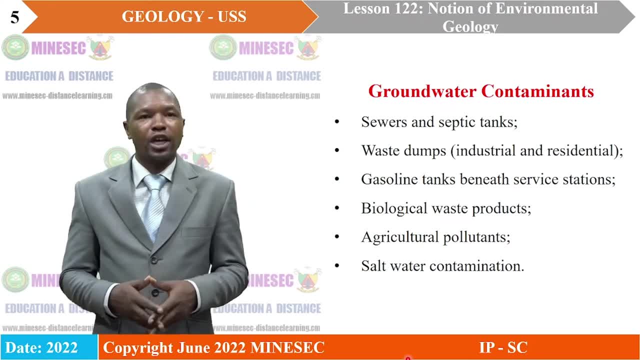 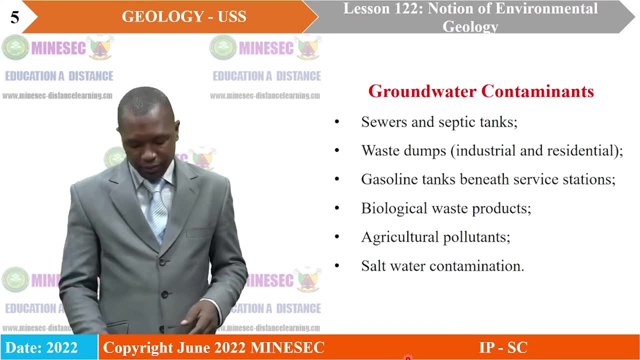 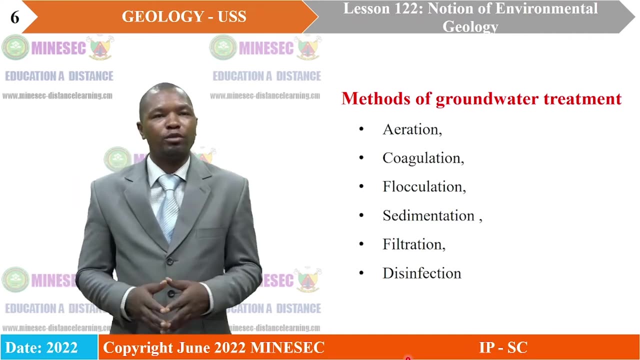 We have agricultural pollutants and we have salt water contamination. Those are the different groundwater contaminants or pollutants. The last part of the question requires that we should just outline the methods of groundwater treatment or of water treatment, because, we said, water treatment has to be a good thing. 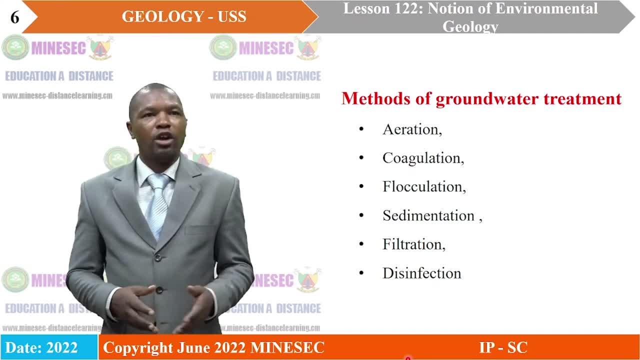 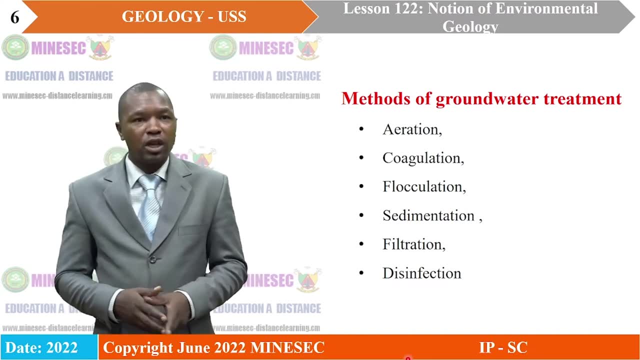 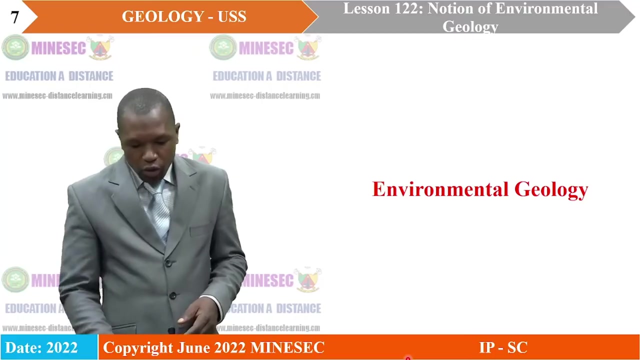 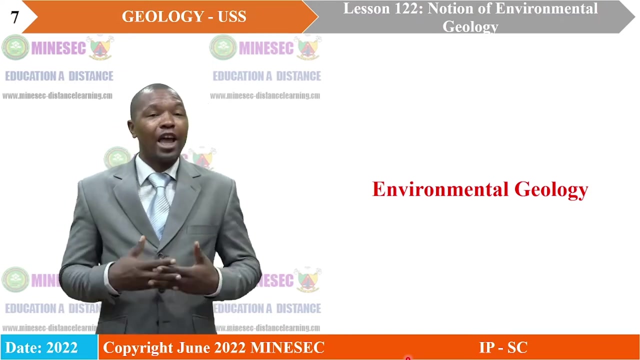 So if we had to do it, we have now only this much water. Its quality has to be down to about 70 percent- really much better than data shows. We also had the geology. after having gone through hydrogeology, it is time to concentrate on the environment. 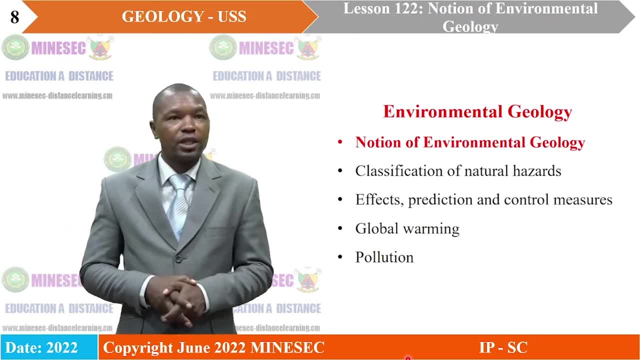 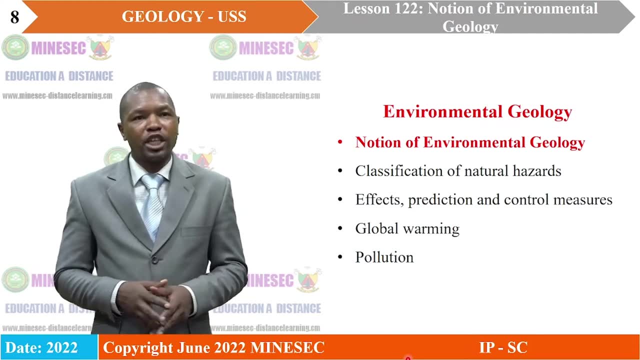 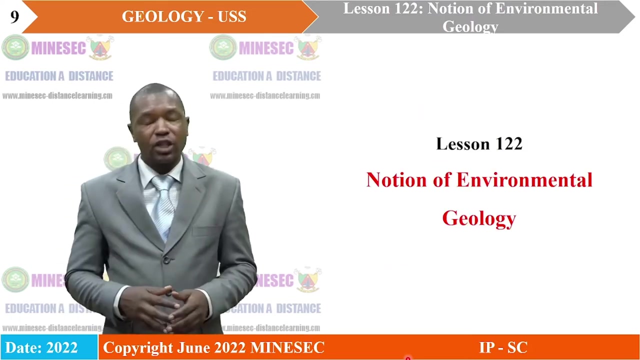 now environmental geology covers notion of environmental geology, classification of natural hazards, effects, prediction and control measures of natural hazards in global warming and pollution. so today we are going to concentrate on notion of environmental geology, so our lesson 122 is titled notion of environmental geology. 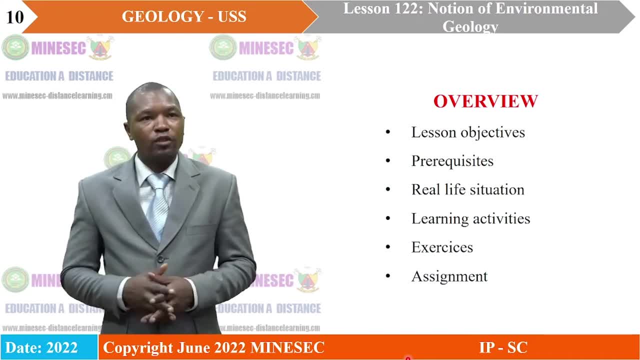 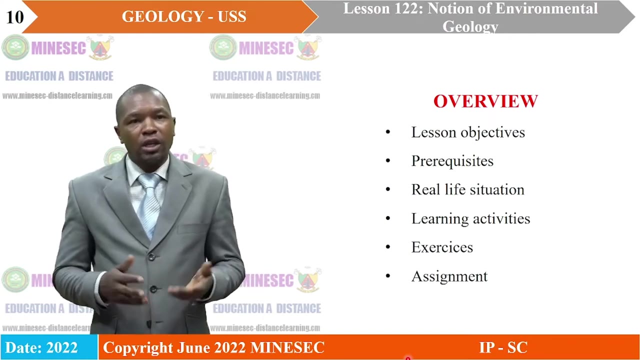 we will look at lesson objectives, come out with some knowledge that is vital for understanding the notion of environmental geology, and then we will come up with our real life situation, carry out some learning activities, come up with some application exercises and end our lesson with an assignment. 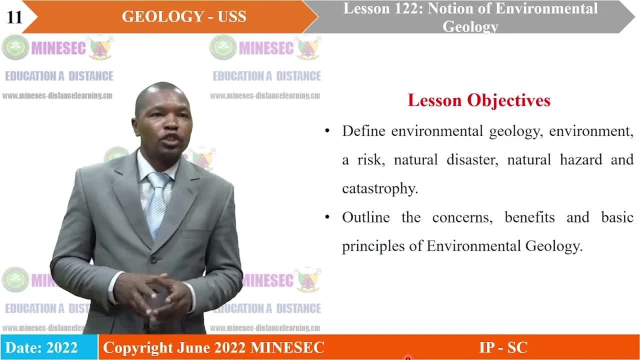 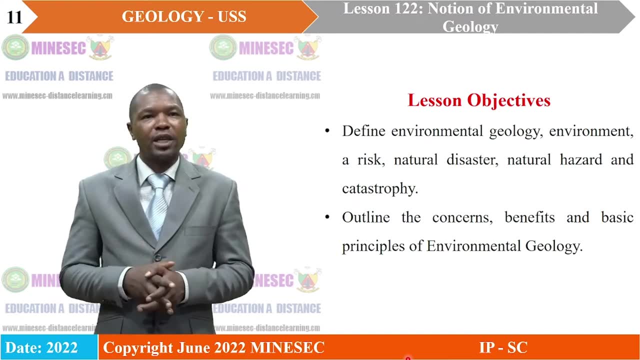 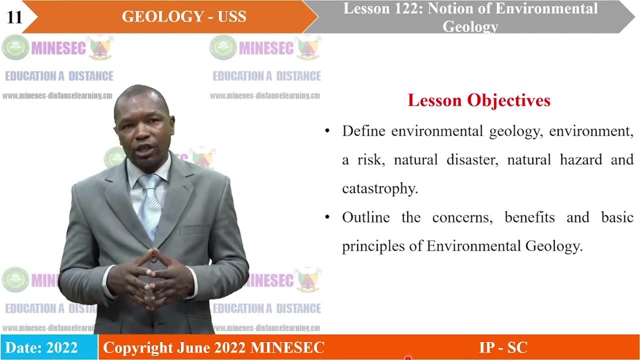 so in our lesson objectives we're going to define environmental geology, define an environment, define a risk, define a natural disaster, define natural hazard and catastrophe. we will also outline the concerns, benefits and the basic principles of environmental geology, the reason why our definitions of risks, natural disasters and natural hazards. 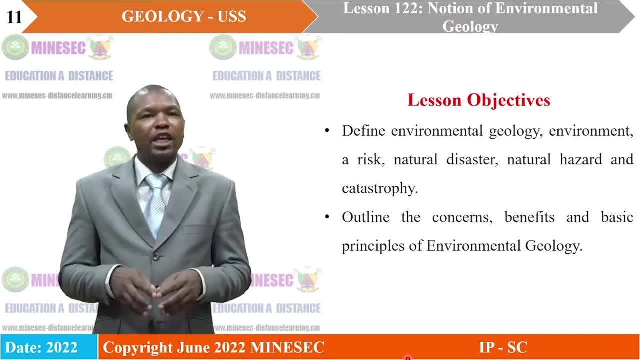 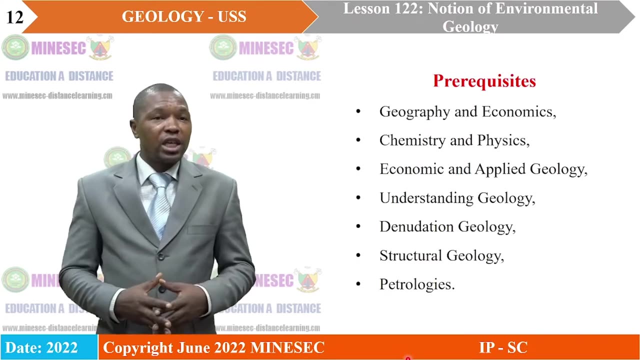 as well as catastrophes. these are things that play in the environment and it is important that in the notion of environmental geology we grabs it so that we don't only get the possible part of it and forget the negative part of it. so knowledge that is very essential for us to have a better understanding of the concept of environmental. 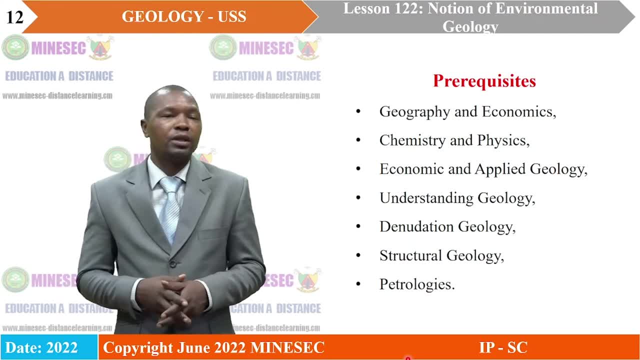 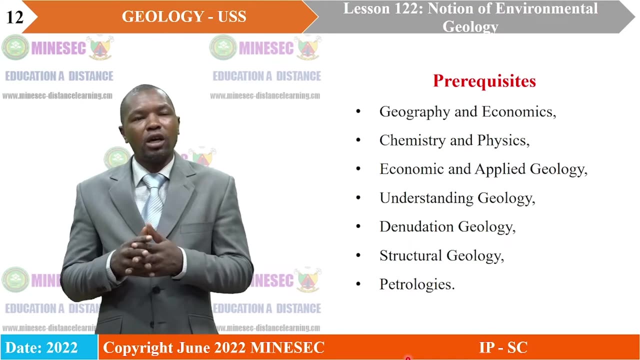 geology will involve knowledge from geography and economics, knowledge from chemistry and physics, knowledge from economic and applied geology, knowledge from understanding geology, then knowledge from denudation geology, and then knowledge from tectonics and structural geology. 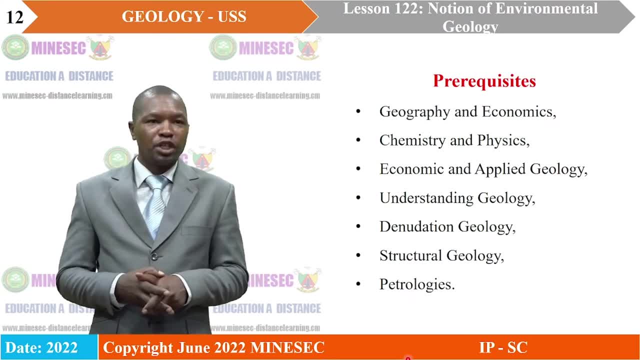 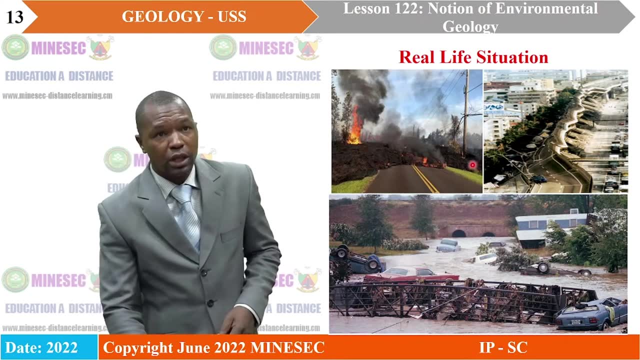 and then, most of all, knowledge from petrologies In our real-life situation. we shall observe these photos. Look at the first photo. You will see there a volcanic event with so much of volcanic materials, released gases, released smoke, Then you have an earthquake situation. 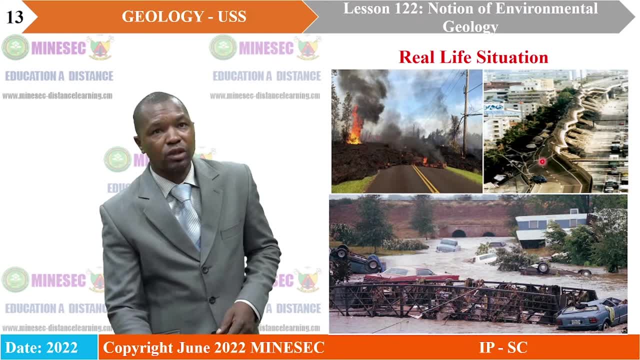 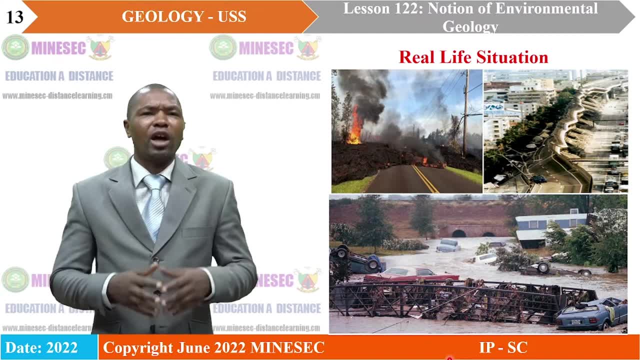 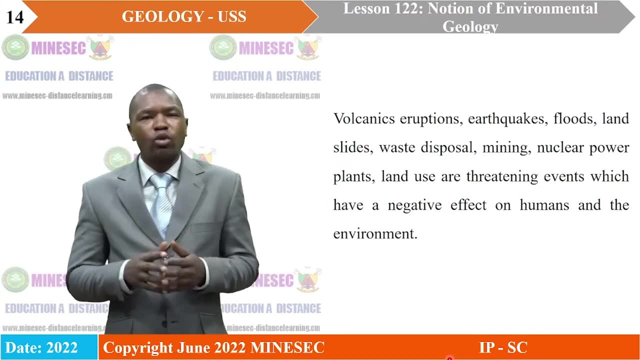 Okay, Okay, Okay, Okay Okay. It's cause. So when you look at these elements, you will realize that our environment is sick. So volcanic eruptions, earthquakes, floods, landslides, waste disposal, mining, nuclear. 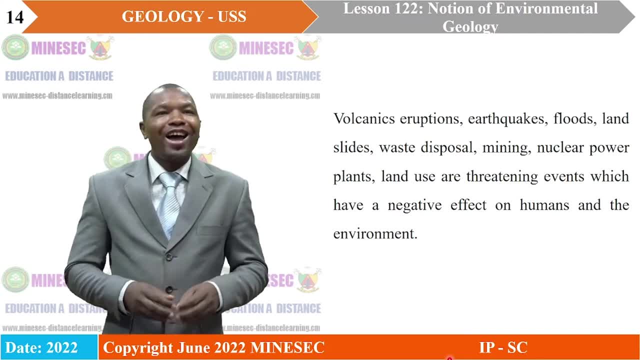 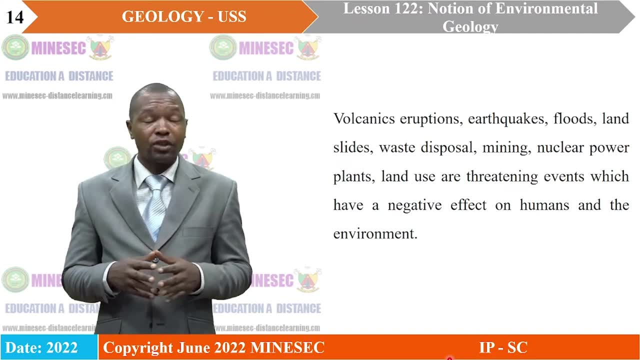 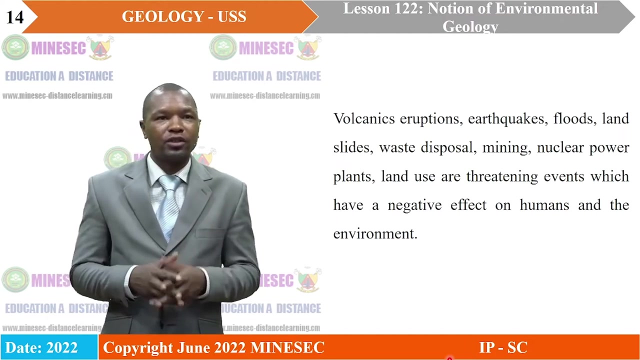 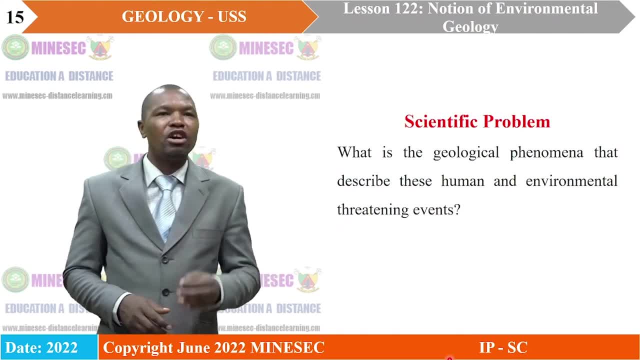 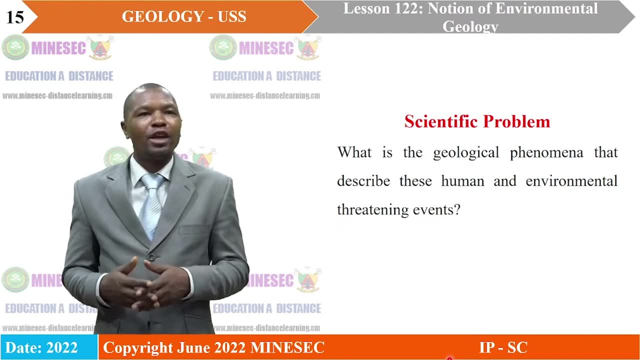 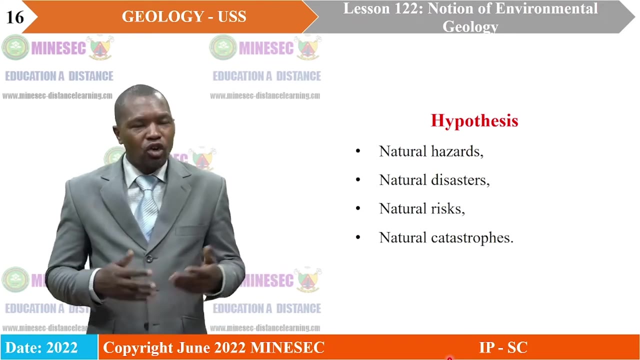 So our problem is: what is the geological phenomenon that describes these human and environmental threatening events? Do we describe them as natural hazards, Or we describe them as natural disasters Or natural risk, Or we describe them as natural catastrophes? As we explore the content of our lesson, we shall come to realize which of the following is true. 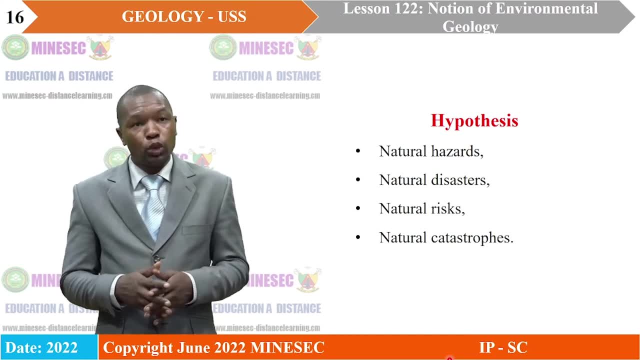 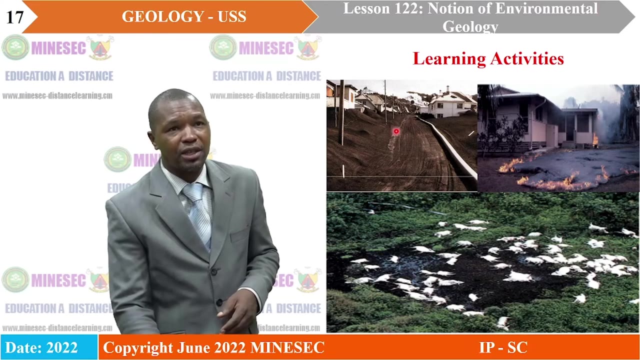 Which of these phenomena can best be used to describe the different elements that affect humans or that are a threat to humans and the environment. So in our learning activity, again you go through these photos, you will realize that this is a portion of a city that has been covered by pyroclastic materials. 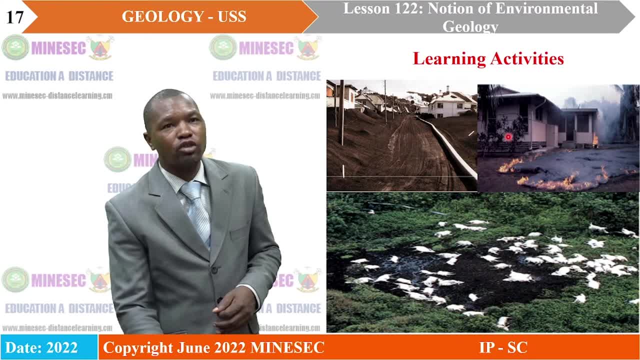 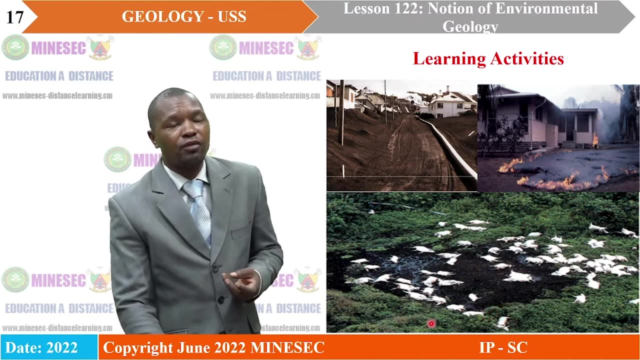 And then you see lava flow here as it goes up to this building. It has set the building on fire due to a lot of heat from the lava. And then you see again from a volcanic source. animals are dying. Probably they would have inhaled a lot of poisonous materials or gases from the volcanic event. 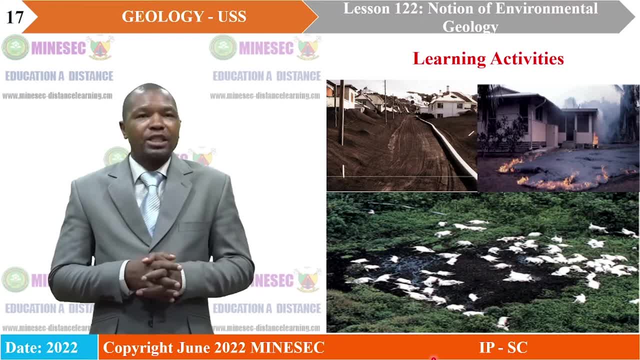 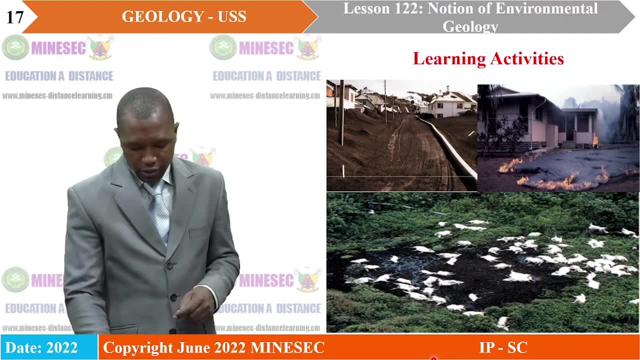 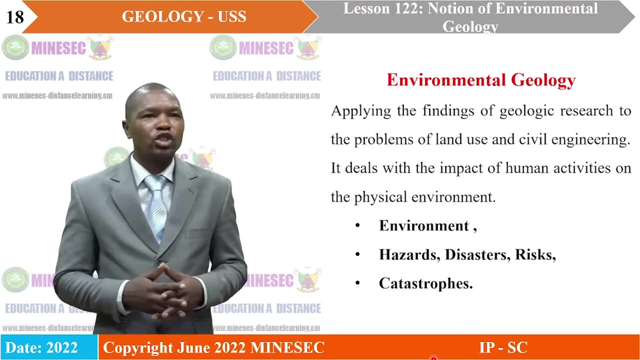 So that is to tell you that volcanic activities can be dangerous to the environment and to organisms, not just humans. So that introduces us to environmental geology. What is it all about? Environmental geology is applying the findings of geologic research to the problems of land use and civil engineering. 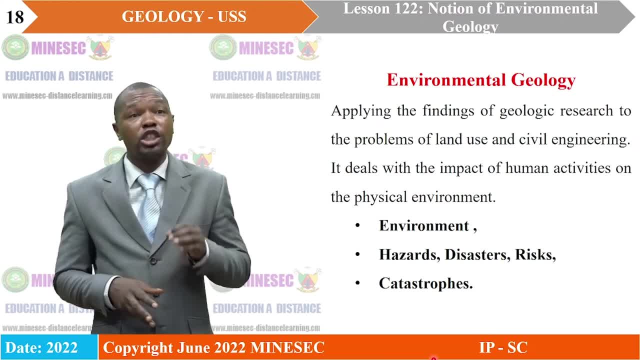 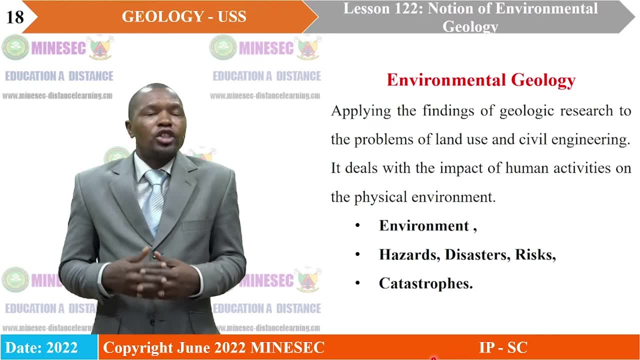 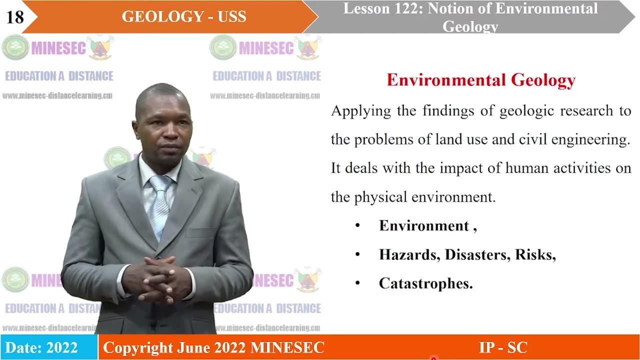 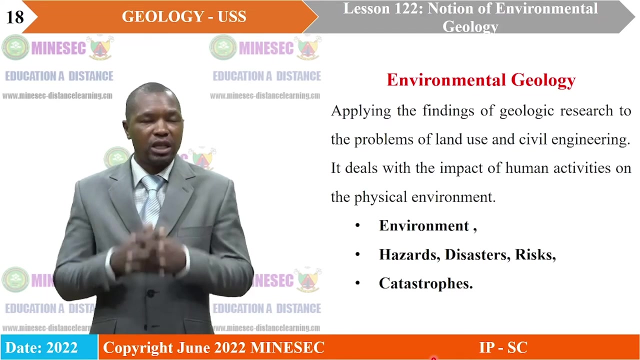 Worth noting is the fact that environmental geology deals with the impact of human activities on the physical environment, Not just the impact of natural disasters, Not just the impact of human activities, But the impact of what Natural events. So that is why we have to understand environmental geology as applying the findings or the knowledge of geologic research to the problems of land use and civil engineering. 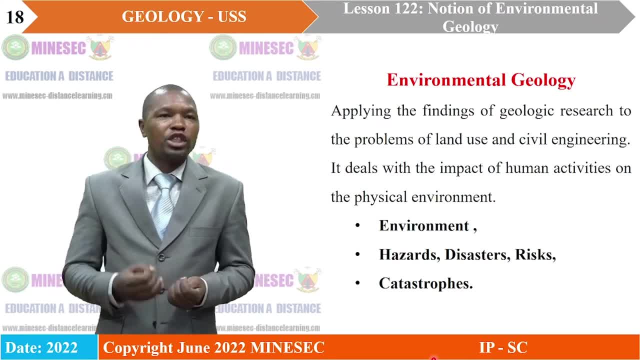 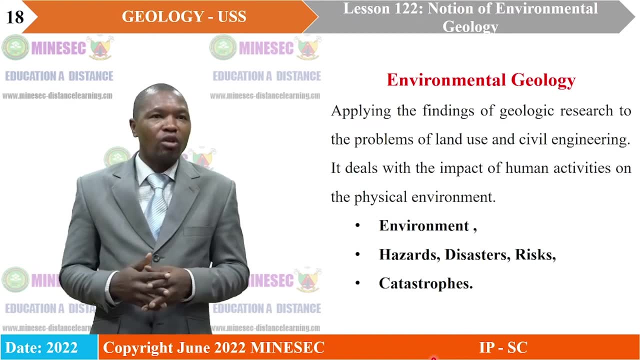 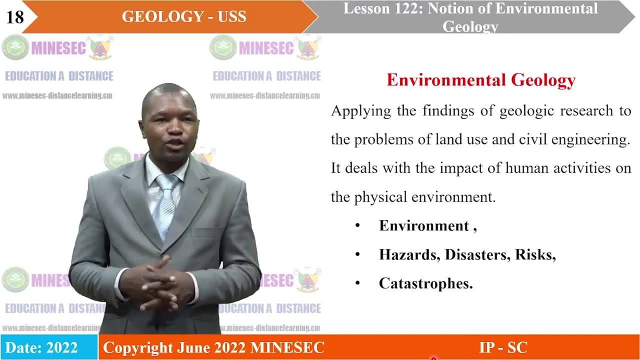 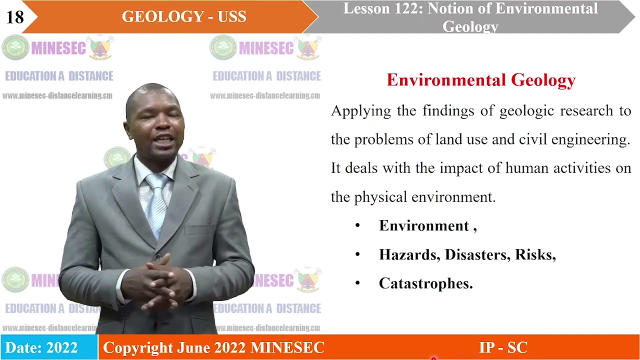 So under environmental geology we shall find out the meaning of the environment. We shall also find out those events which come through: hazards, disasters, risk and catastrophes. So we will want to understand what an environment is, what hazards are, what disasters are, what a risk is, what catastrophes are. 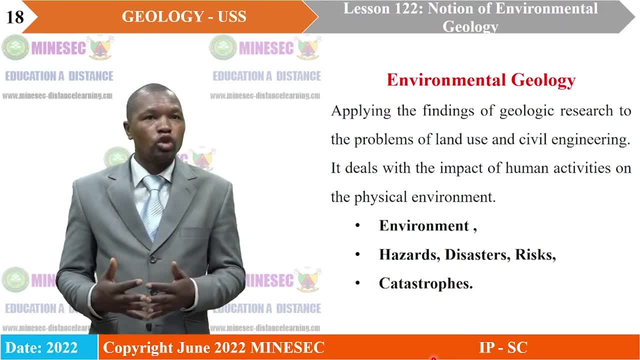 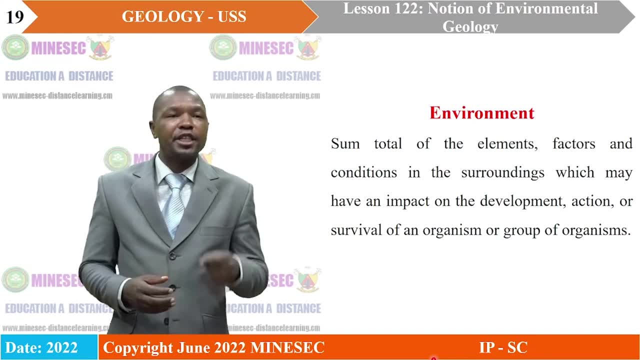 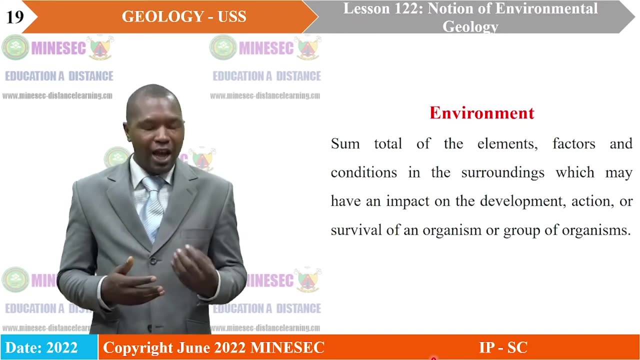 As we go through the notion of environmental geology, Now An environment. An environment is the sum total of the elements, factors and conditions in the surroundings which may have an impact on the development, action or survival of an organism or group of organisms. 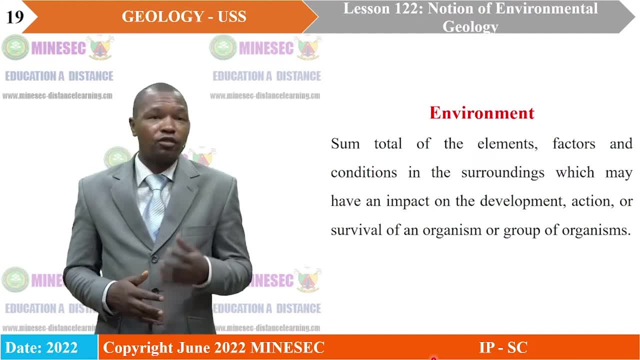 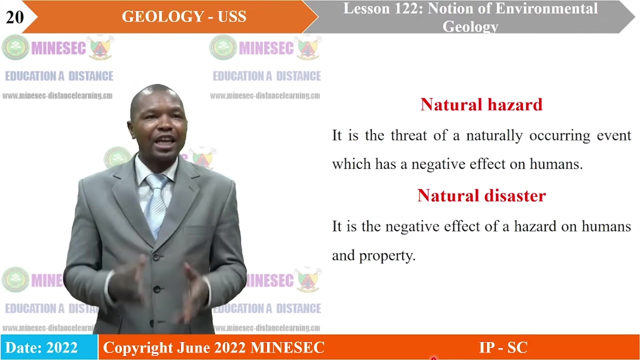 So again, environment is the sum total of the elements, factors and conditions in the surroundings which may have an impact on the development, action or survival of an organism or group of organisms. What is a natural hazard? A natural hazard is the threat of a naturally occurring event which has a negative effect on humans. 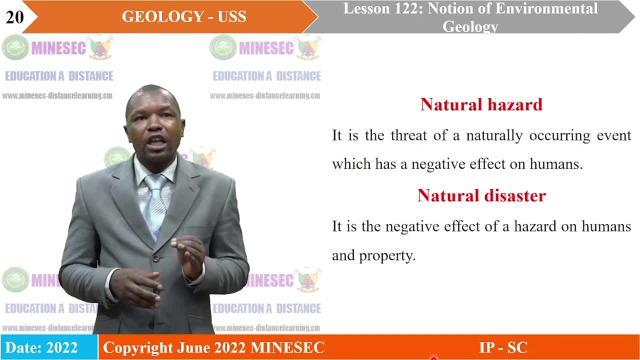 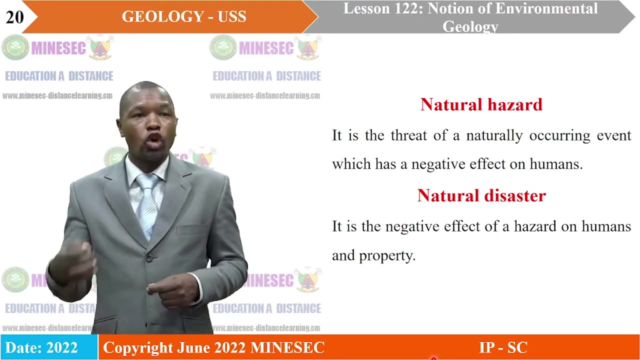 A natural hazard is the threat of a naturally occurring event which has a negative effect on humans. A natural hazard is the threat of a naturally occurring event which has a negative effect on humans, While a natural disaster is the negative effect of a hazard on humans and property. 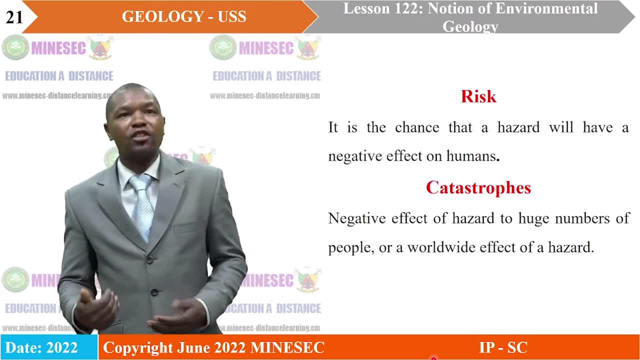 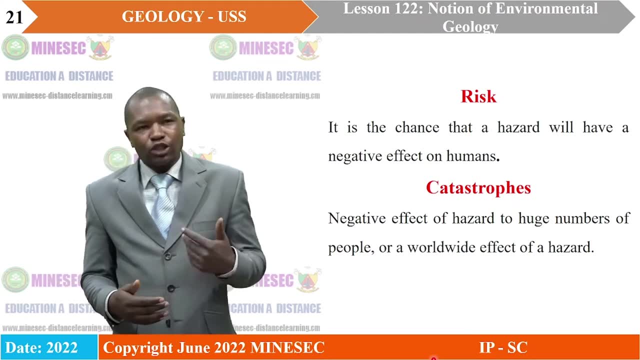 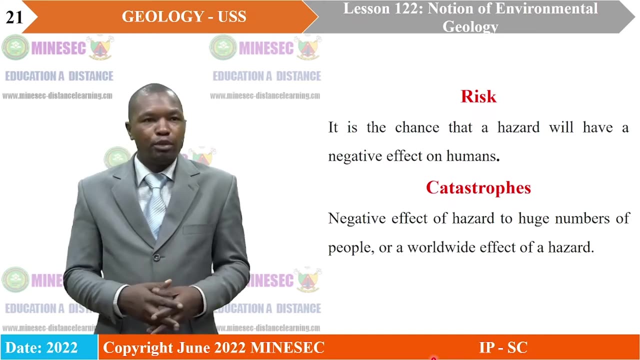 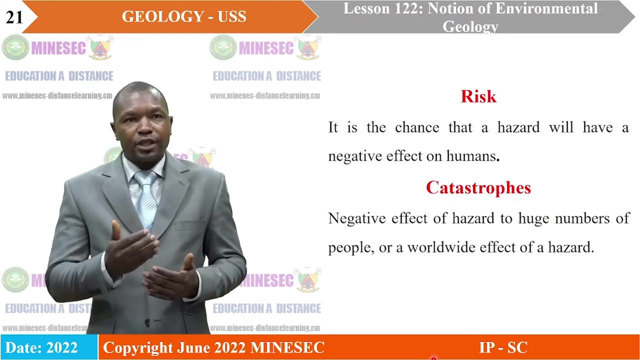 Then a risk is the chance that a hazard will have a negative effect on humans. A catastrophe is a negative effect of a hazard to huge numbers of people or a worldwide effect of a hazard. So you see that risk, disaster, catastrophe- all centers around the event called hazard. 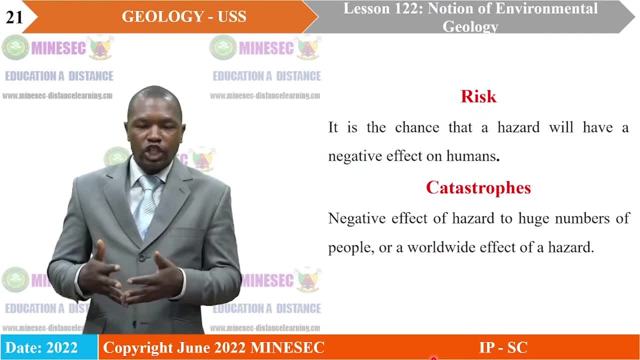 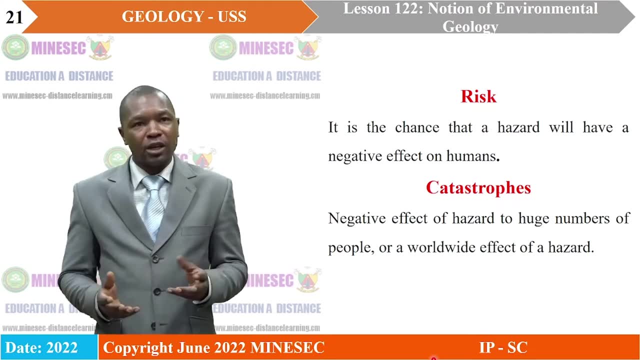 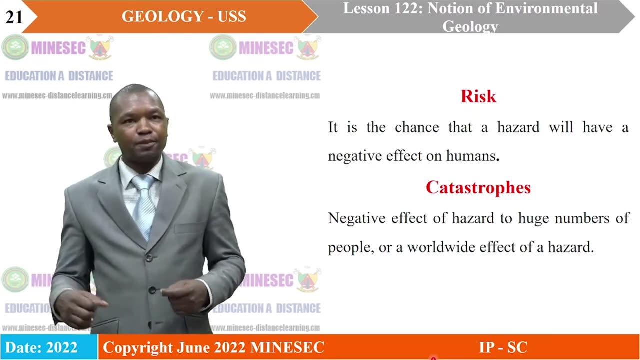 This is to help us understand the nature of the problem we evoked at the beginning of our lesson. So here the whole phenomenon is titled hazard, whereas the effect, when negative, we call it a disaster. When the chance that the event will have a negative effect is a risk. 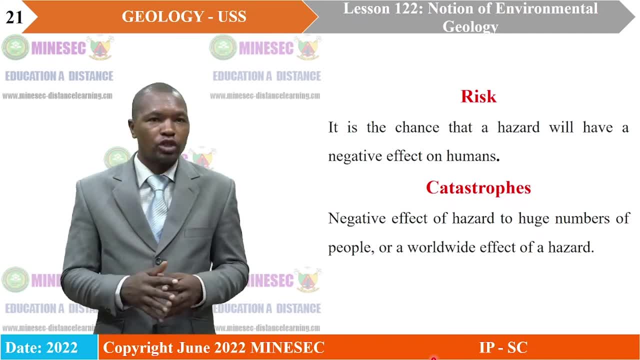 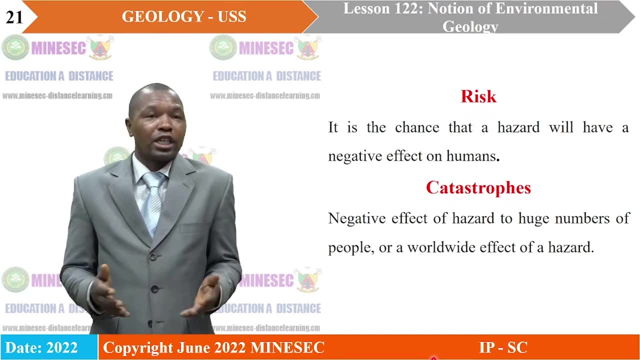 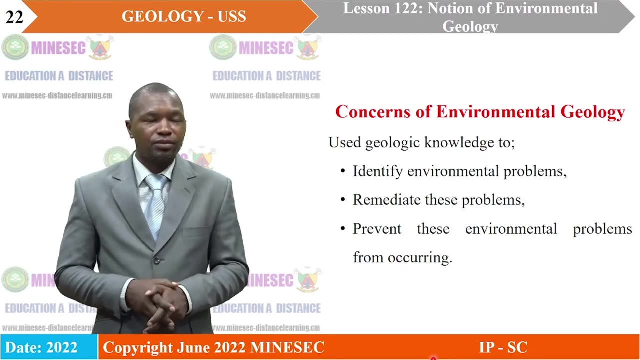 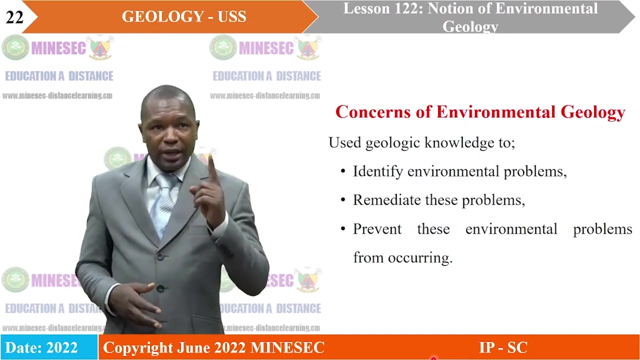 and then, when the effect is just so much on a large number of people, or when it is a worldwide kind of effect, then we call it catastrophe. Now, what are the concerns of environmental geology? Now, environmental geology uses geologic knowledge to one identify environmental problems. 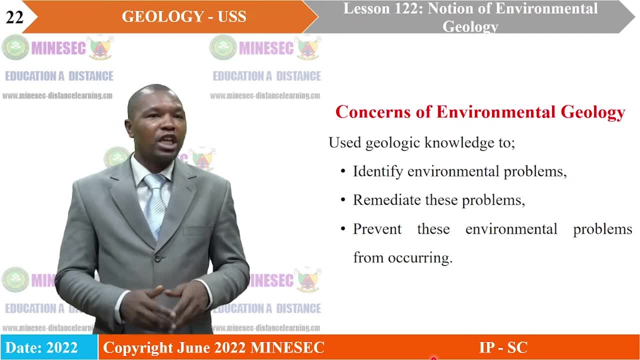 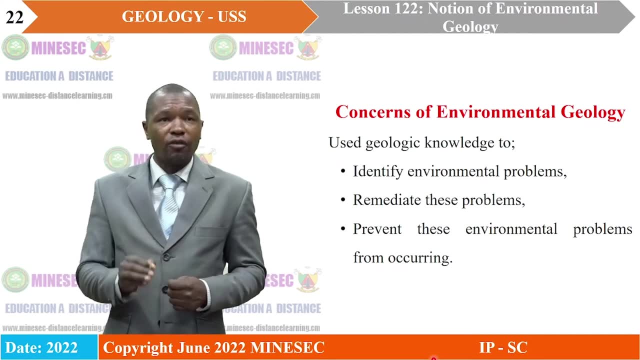 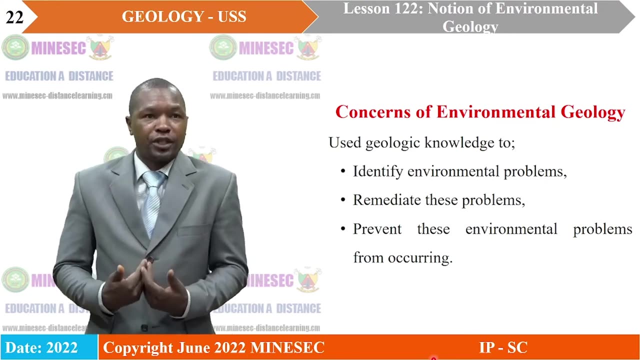 two remediate these problems and then three prevent these environmental problems from occurring. So the concerns of environmental geology are three in number. We could equally say the concerns. The concerns of an environmental geologist would be to use their knowledge of geology. 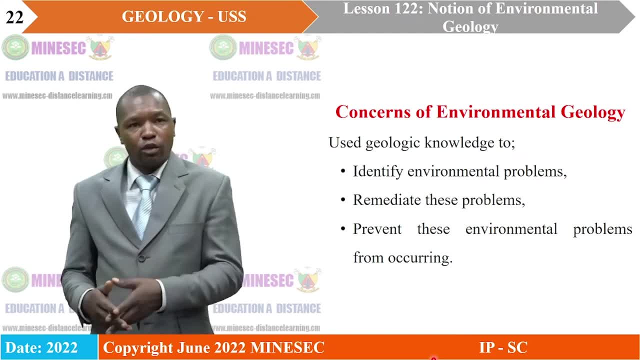 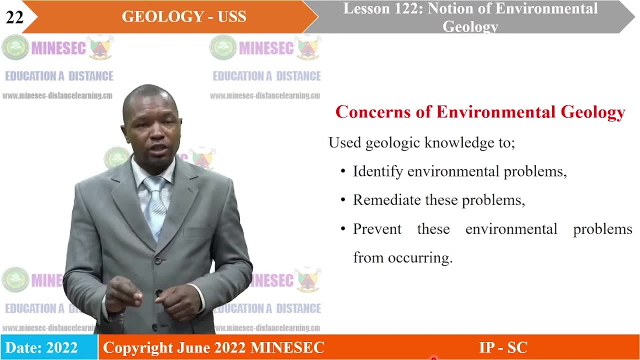 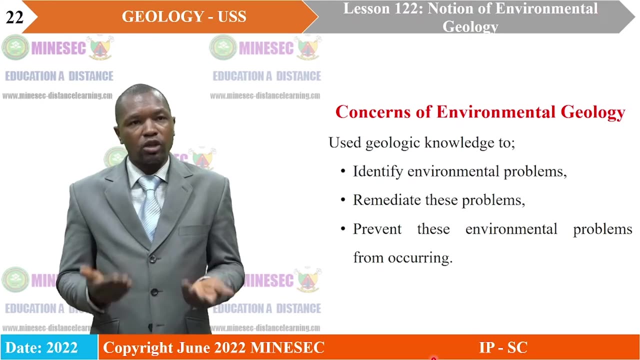 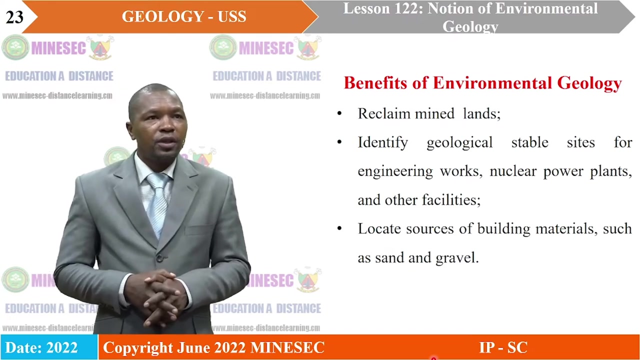 to identify environmental problems, remediate these problems and then prevent these environmental problems from occurring. Those are the concerns of what an environmental geologist or environmental geology is supposed to concentrate on. What about the benefits of environmental geology? Is it worth studying it at all? 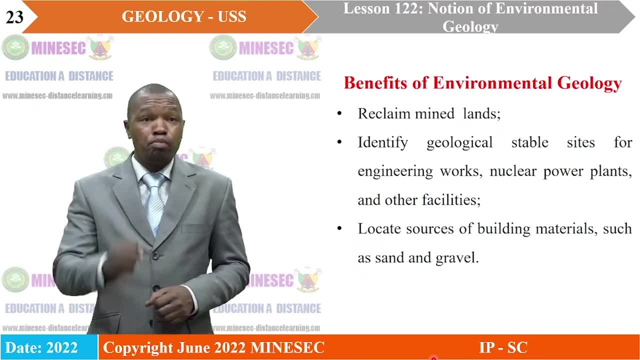 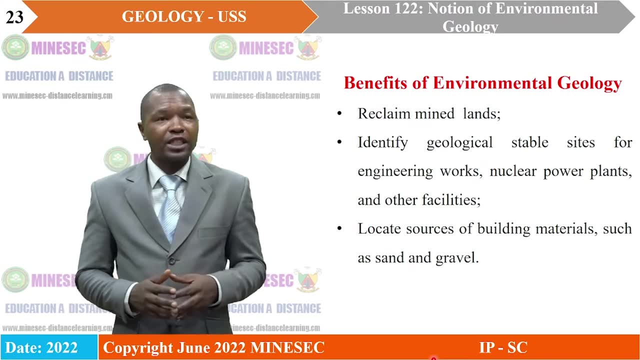 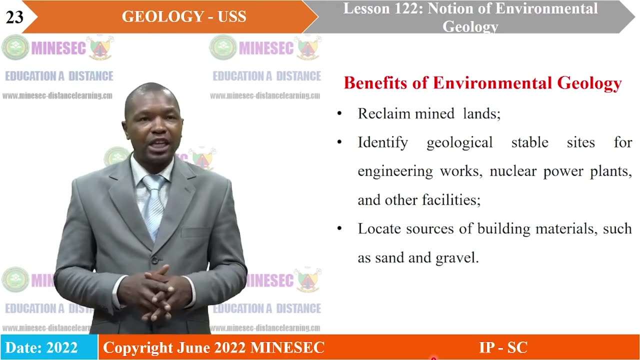 Now, the benefits of environmental geology push us to concentrate on this particular aspect of geology. One, the fact that the first benefit is what? To reclaim? mined lands, That is, mine rehabilitation. You see situations where a mining work has been done. 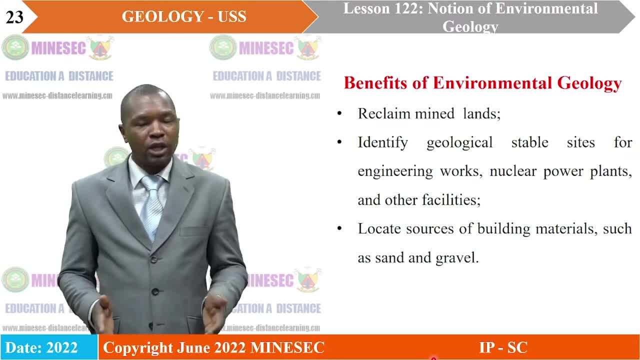 or materialization Materials have been extracted somewhere and the area is abandoned. Water stands in that area and becomes breeding grounds for mosquitoes. You can also see escapements that have been allowed after materials have been extracted, and then soon it becomes what? 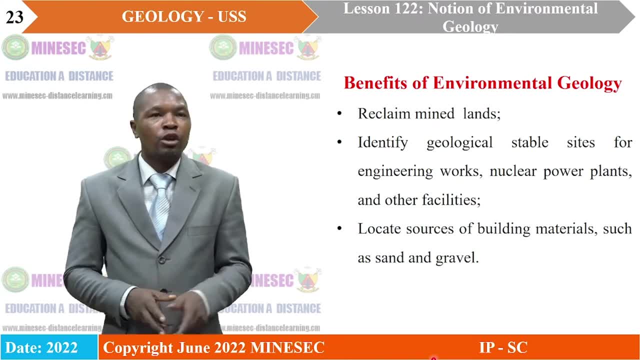 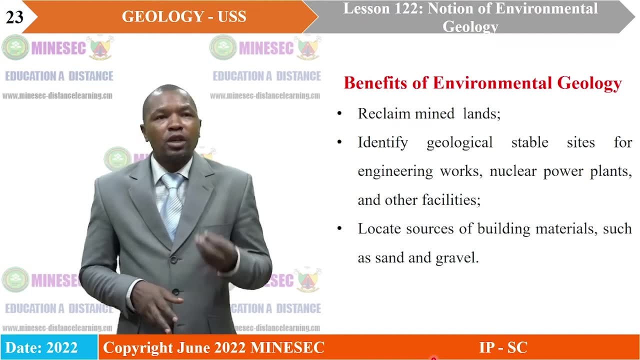 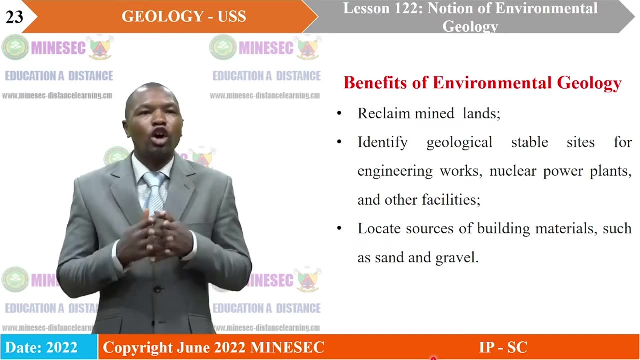 A problem, a threat to the people in the area. So one of the benefits of environmental geology is to reclaim those mined sites. Then it is also to identify geological stable sites For engineering works, nuclear power plants and the other facilities. 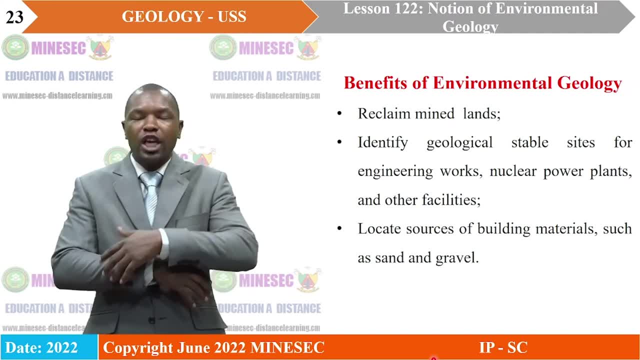 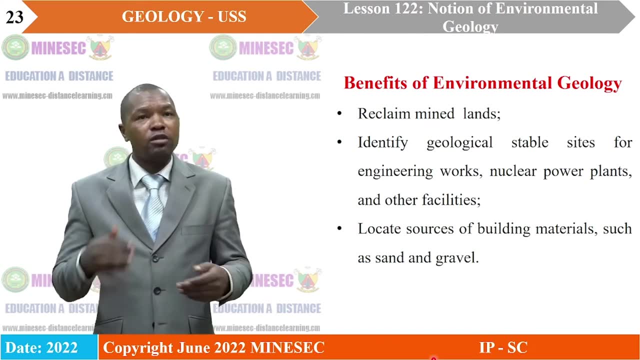 In order to do a construction, there must be work, research, work geologically oriented, in order that effective information is given before sites are located for engineering works or for construction works or for power plants and other facilities. That has to do with the use of materials, especially what it has to do with construction works. 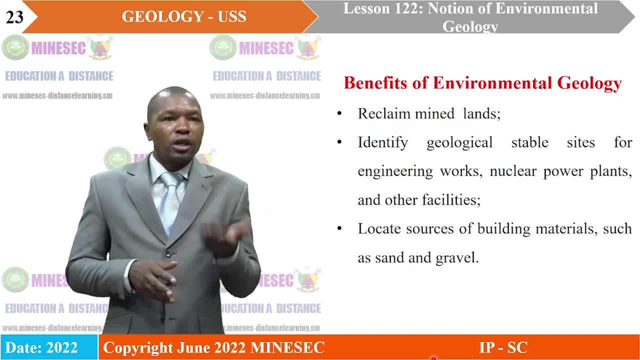 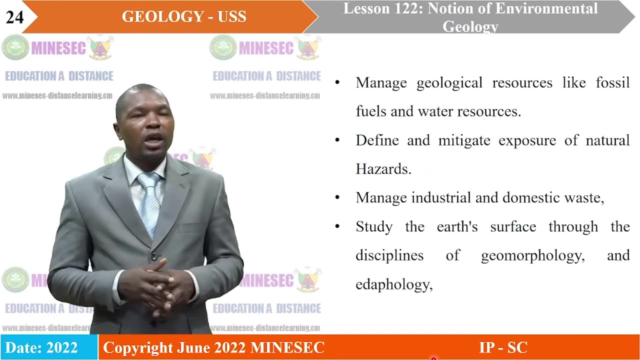 Then environmental geology is also beneficial, since through it we locate sources of building materials such as sand and gravel. More benefits: it guides to manage geological resources like fossil fuels and water resources. It also helps to define and mitigate exposure of natural hazards. 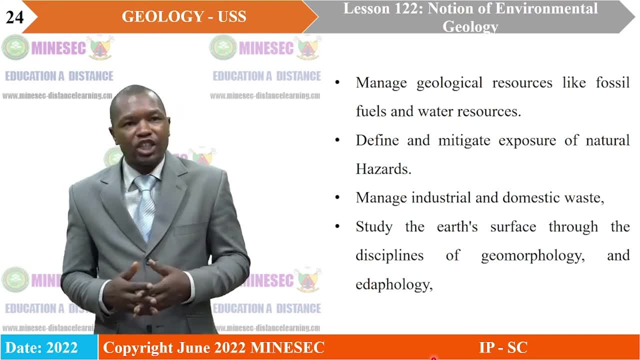 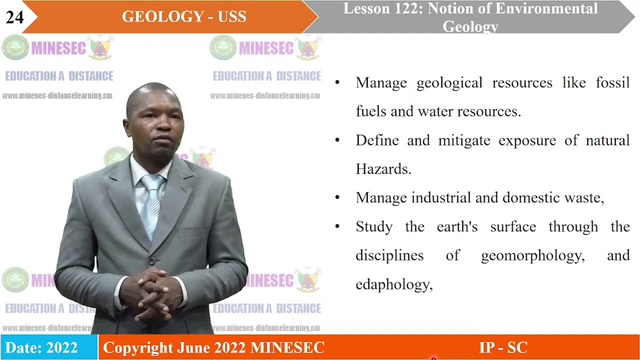 Then it helps to manage industrial and domestic waste or residential waste, Very important here. In communities where you know there is no direct influence of environmental geologists, what happens is that waste is dumped anyhow. You even find some dumped right at the road sites. 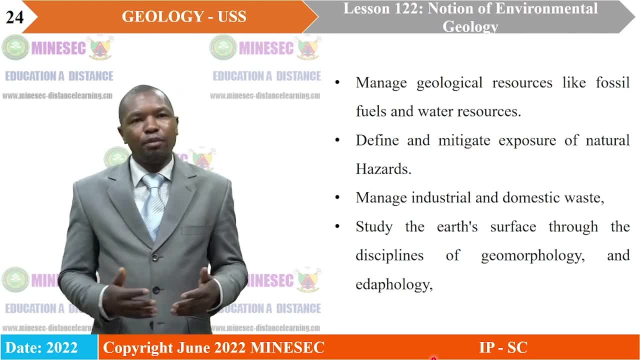 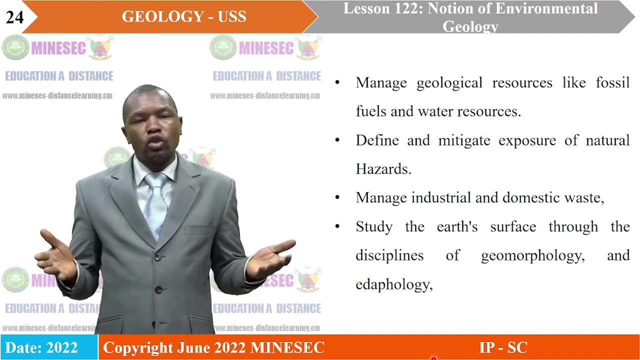 People passage passages are destroyed. People passages are destroyed. People passages are destroyed. People passages are destructed. People cannot be comfortable because of the sand that will come from such, and then leakages from such materials will go to other amenities that are useful, making life dangerous. 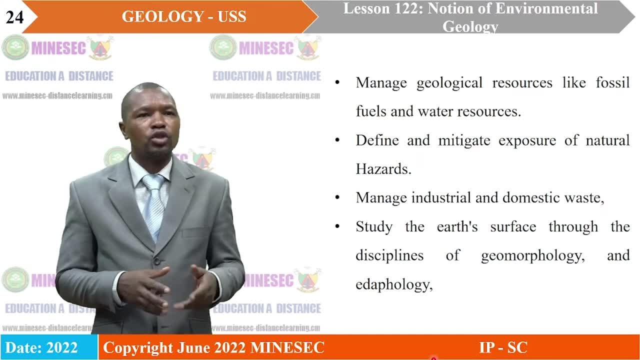 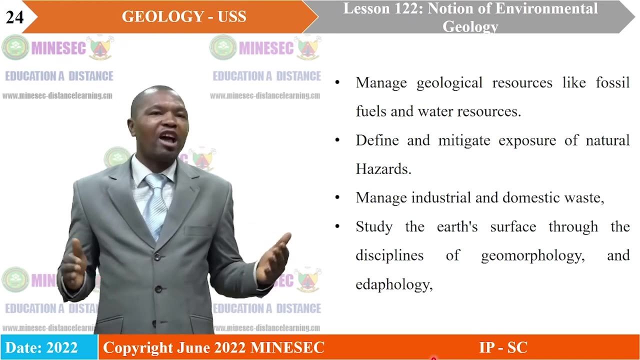 Environmental geology also helps to study the Earth's surface through the disciplines of geomorphology and edaphology. These are areas, areas that we have to guide on how the morphology of the earth's surface looks like: Areas where water concentrates, areas where there are hills, areas 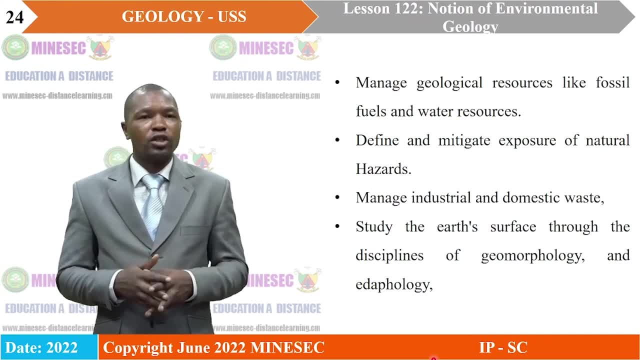 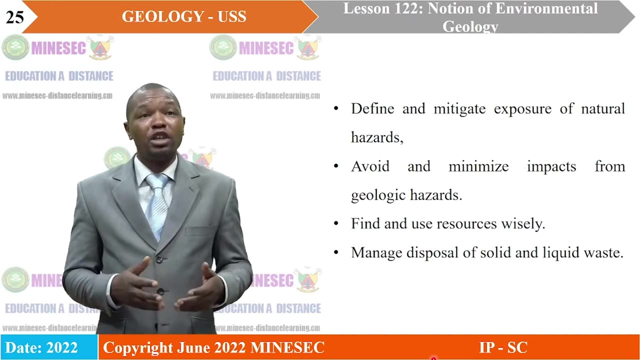 where there are a lot of instability because of landslides and so on. This knowledge is required and it can only come from environmental geologists. More so, environmental geology guides to define and to mitigate exposure of natural hazards, and to avoid and minimize. 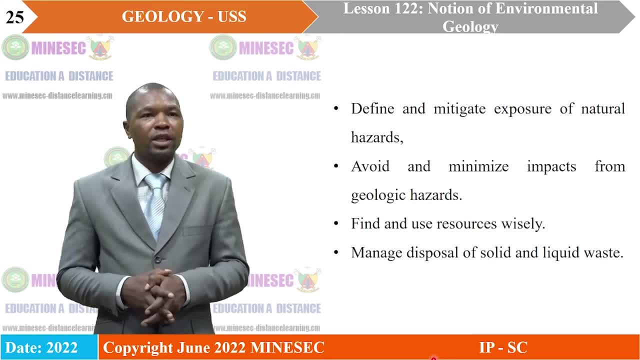 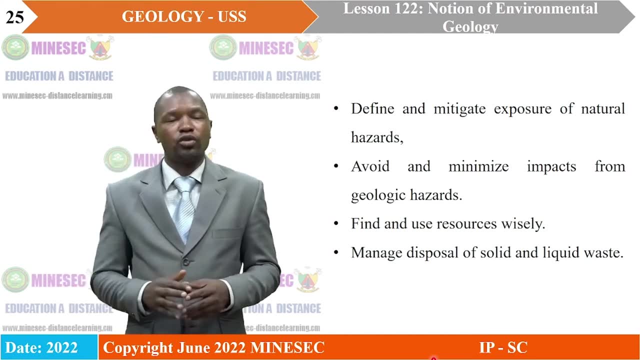 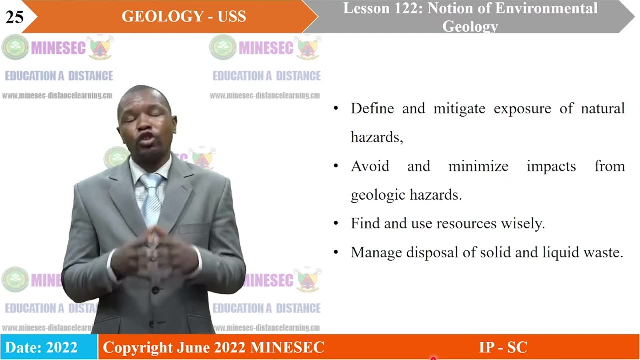 impacts from geologic hazards. It also helps to find and use resources wisely. Here we must concentrate to say that when we come to explorations, especially of our different mines, we must try to define some mining laws that will govern on how the mining is supposed. 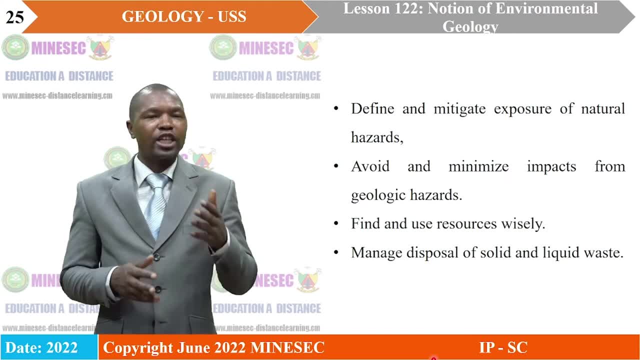 to take place, Permissions are necessary. The way extractions are supposed to be done are necessary. This information can only come from environmental geology. Environmental geology also helps to manage disposal of solid and liquid waste. Very important Solid and liquid waste. 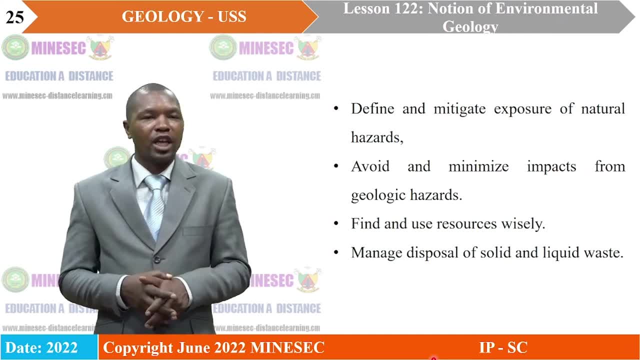 are the most dominant waste that we have in nature. When it has to go to gaseous, it just becomes very challenging. So how to manage solid and liquid waste? We can only have that knowledge through environmental geology. Now. 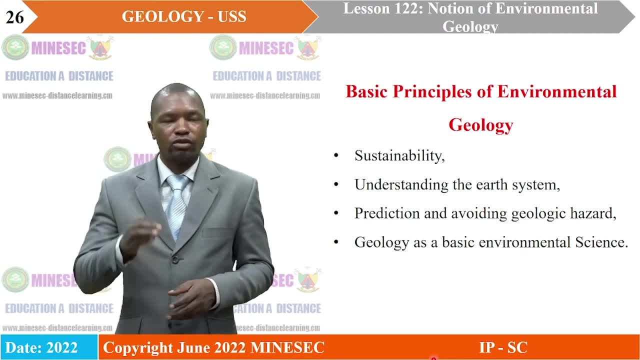 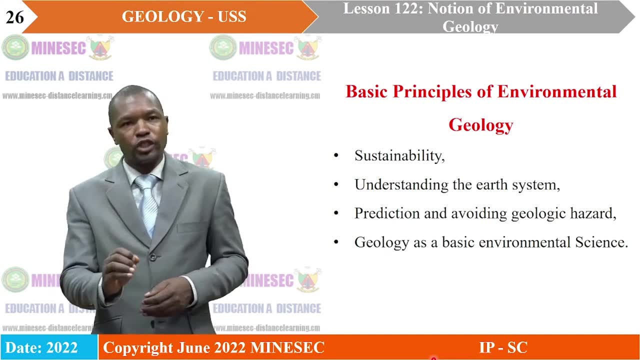 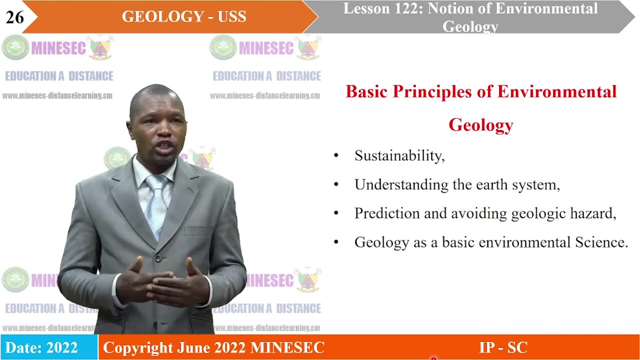 what are the basic principles of environmental geology? What are the fundamentals for environmental geology? The first one is for sustainability. We cannot have an environment where life is not comfortable, So environmental geology is there to create an atmosphere where we can sustainably manage. 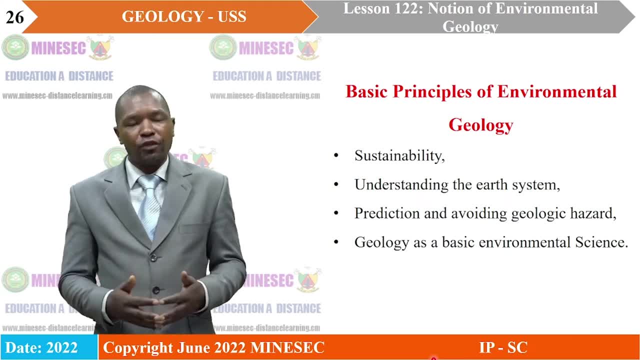 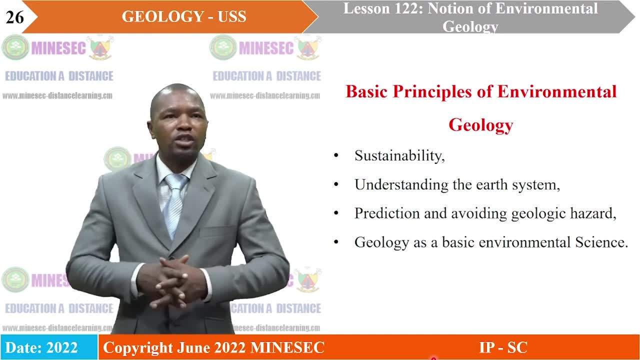 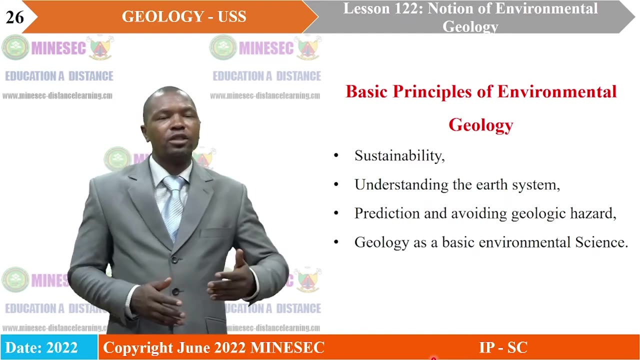 any other thing: Our lives, the different resources that we have in order to make the environment comfortable for everyone. Environmental. the next principle is understanding the earth's system. The earth is a system. You find that you have the atmospheric part of the earth. 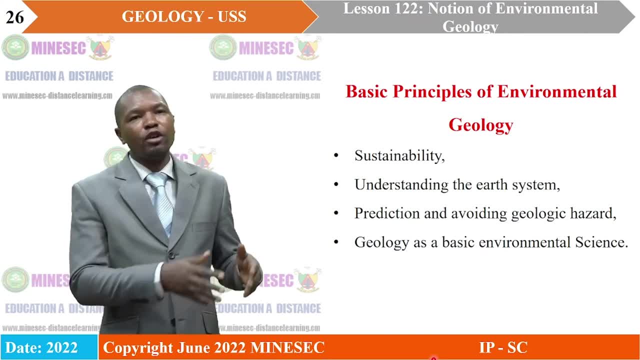 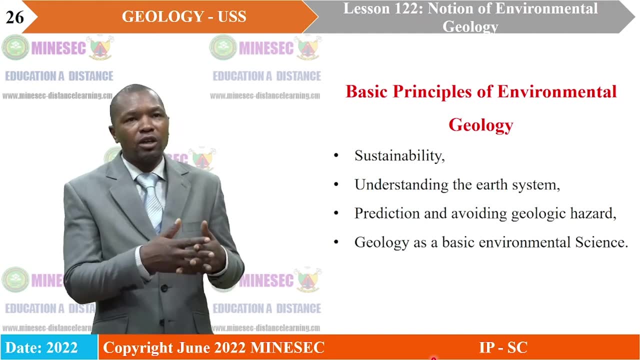 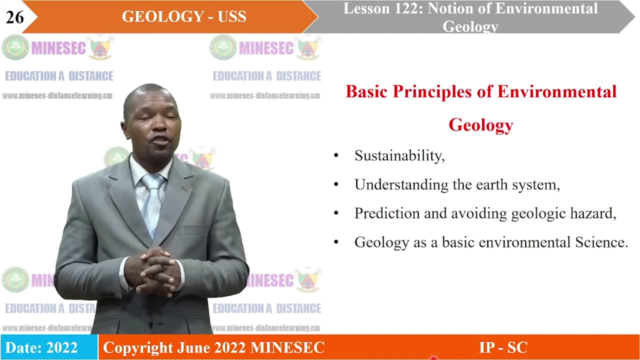 you have the hydrospheric part of the earth, you have the biological part of the earth, you have the lithospheric, you have the, the, the, and then you have the systems of the earth. This way, the environmental geologists, 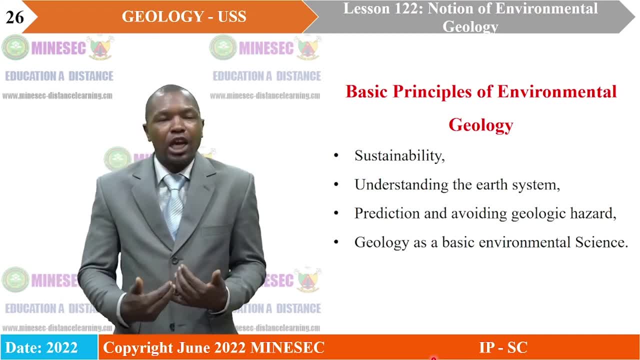 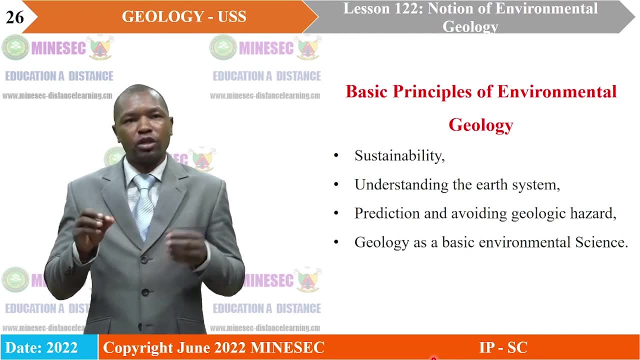 especially with the atmospheric, has to come in in order to treat or to help an understanding of how climatology works. Go by This way: the knowledge. the knowledge is vital so that we know how to place our seasons, We know when there is a rainy season. 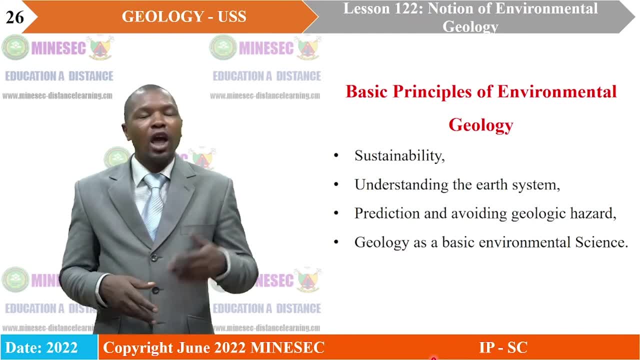 and when in the rainy season there is too much rain, and also how to control weather elements. Then environmental. the next principle is prediction and avoiding of geologic hazards- Very important principle. Then the last one is geology as a basic environmental science. 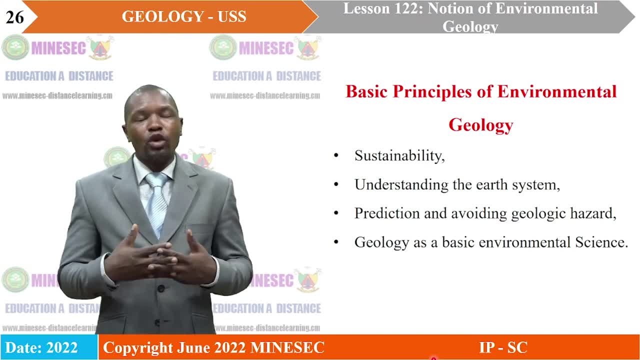 We cannot go without this because without understanding the geological resources that we have in our earth planet, it will be difficult. We will tend to provoke danger to ourselves in the way we go about those geologic resources. So that is one of the principles. 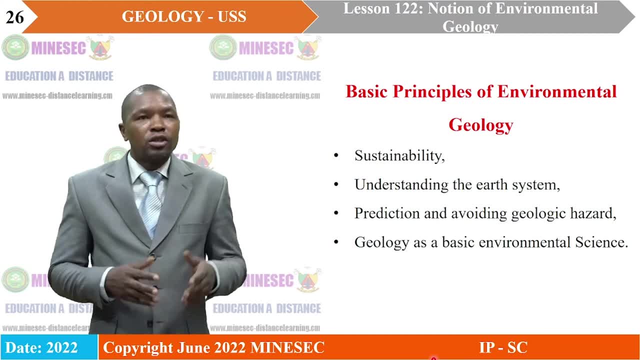 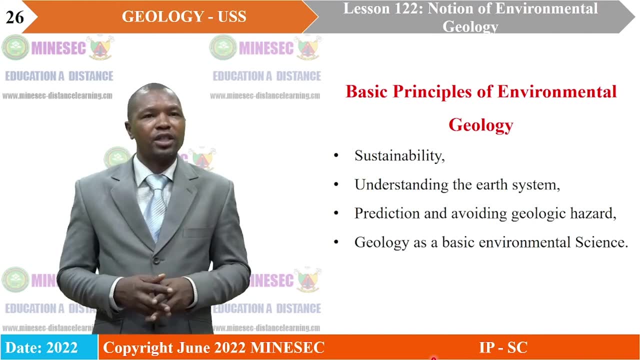 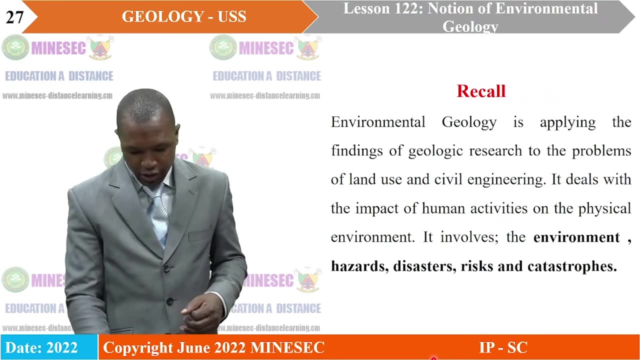 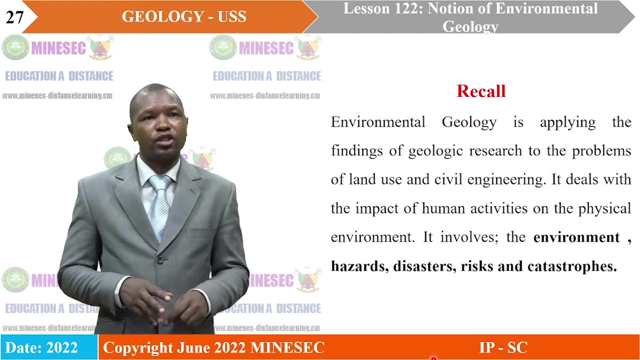 So we generally are saying that Environmental geology has some basic principles: Sustainability is one, understanding the earth system is the other, prediction and avoiding geologic hazards and geology as a basic environmental science. To recall, environmental geology is applying the findings of geologic research. 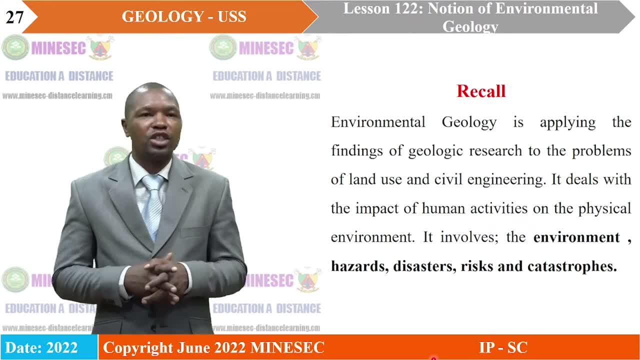 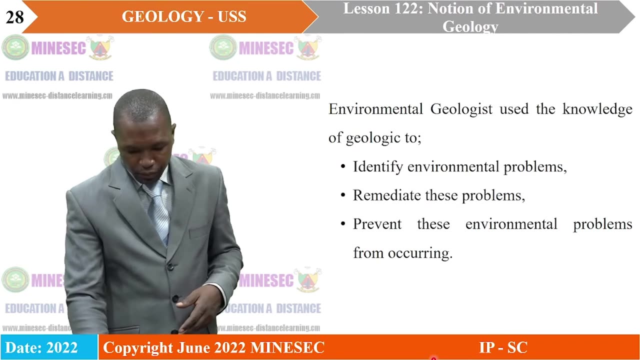 to the problems of land use and civil engineering. It deals with the impact of human activities on the physical environment. It involves the environment, hazards, disasters, risks and catastrophes. Environmental geology uses the knowledge of geology to identify environmental problems. 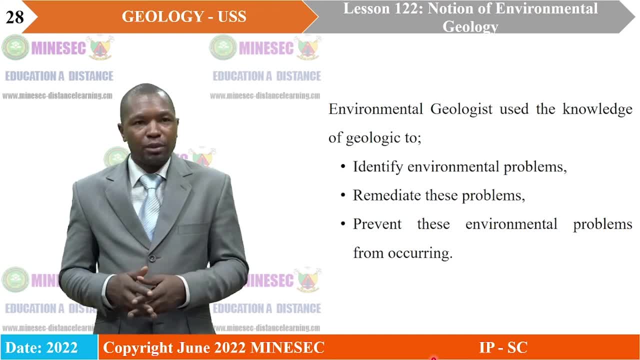 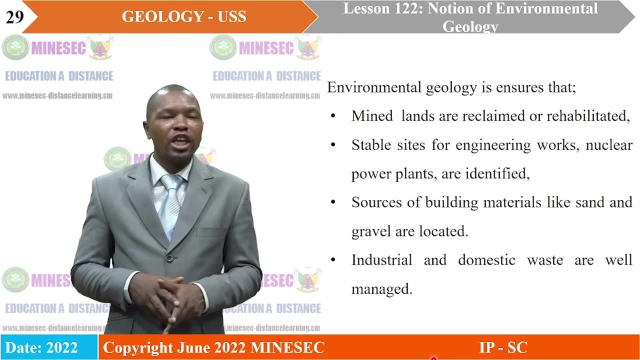 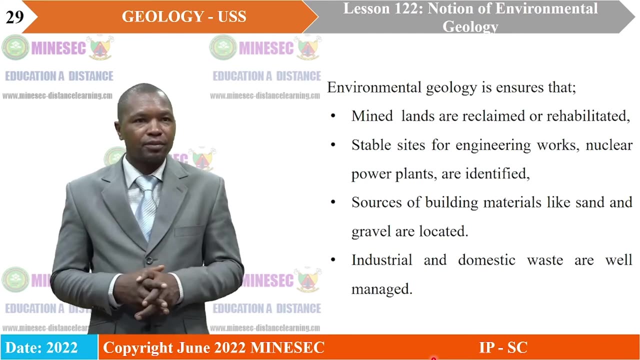 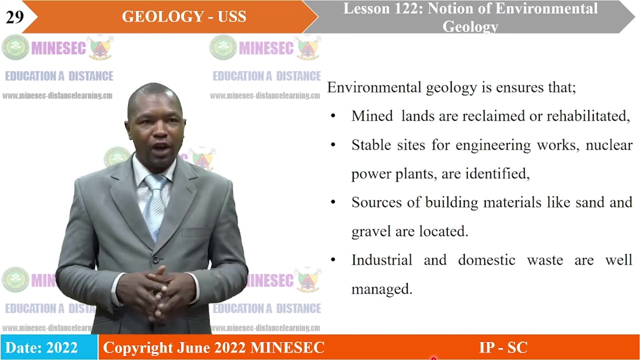 to remediate these problems, as well as prevent these environmental problems from occurring. Environmental geology ensures that mined lands are reclaimed or rehabilitated. It also ensures that stable sites for engineering works- nuclear power plants- are identified. Environmental geology also ensures sources, or ensures that sources. 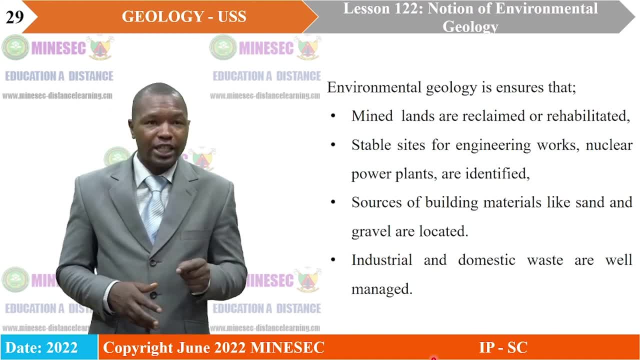 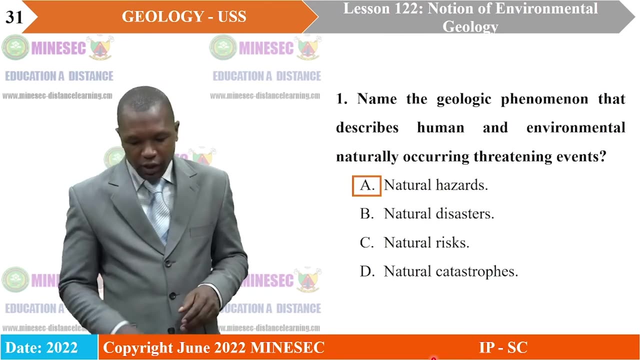 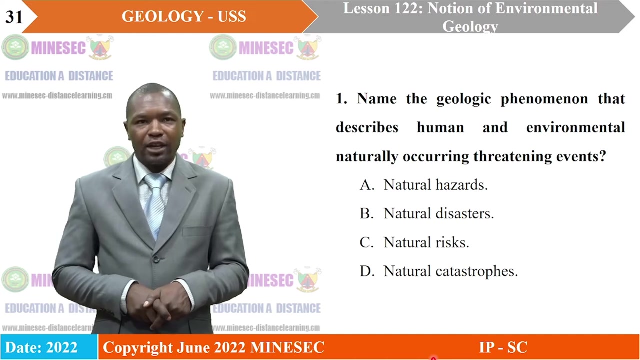 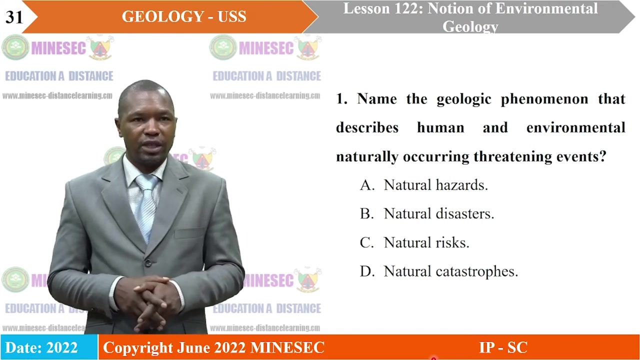 of building materials like sand and gravel are located and well. Environmental geology also ensures environmental sustainability that industrial and the domestic waste are well managed. we dive into some exercises. exercise number one name the geologic phenomenon that describes human and environmental naturally occurring threatening events. you know this. 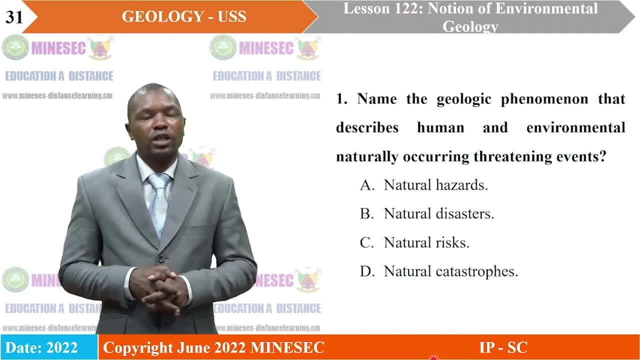 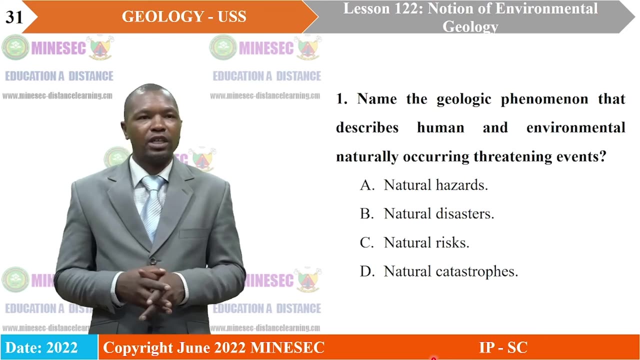 question is related to our today's scientific problem. we evoked at the beginning of the lesson. from going through our lesson, what should be that geologic phenomenon that describes human and environmental naturally occurring threatening events? a natural hazards be natural disasters, see natural risk d natural catastrophes. our correct answer is natural hazards. 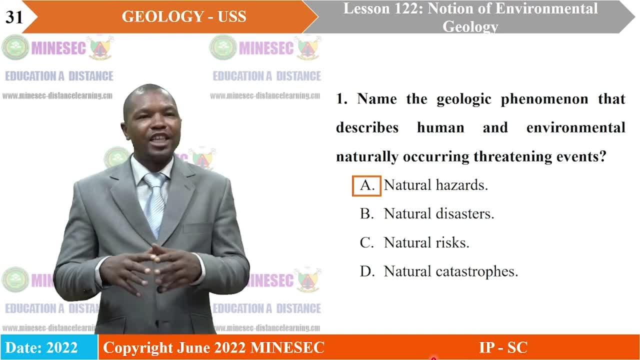 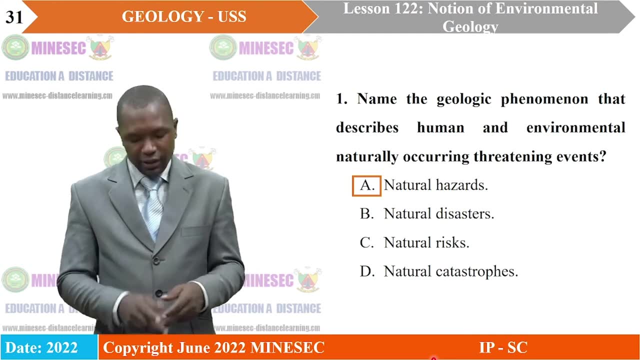 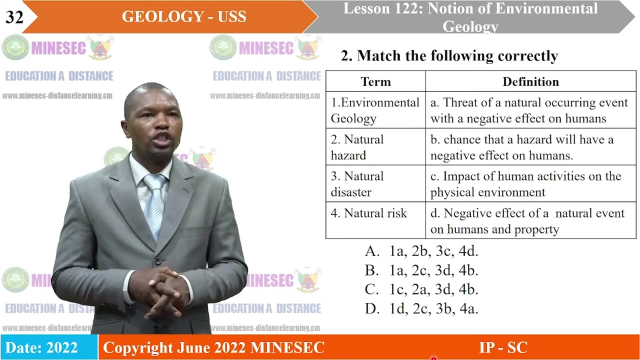 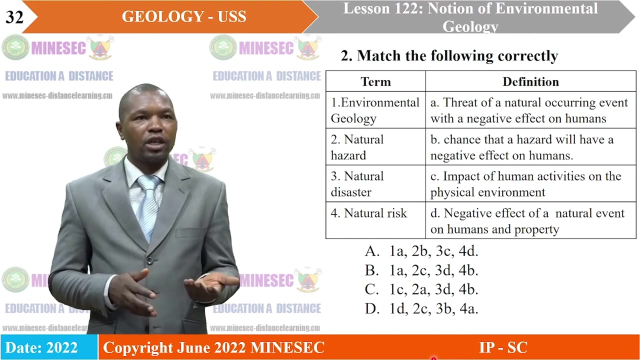 Natural disasters, risks and catastrophes are a description of the consequences of natural hazards, So the phenomenon is natural hazards. Now match the following correctly: You have environmental geology, natural hazards, natural disaster and natural risks. Their definitions are related as follows. 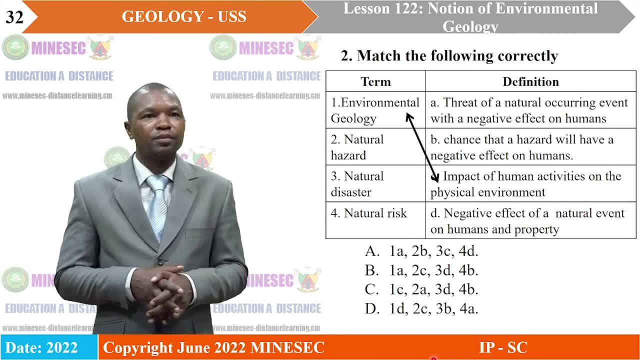 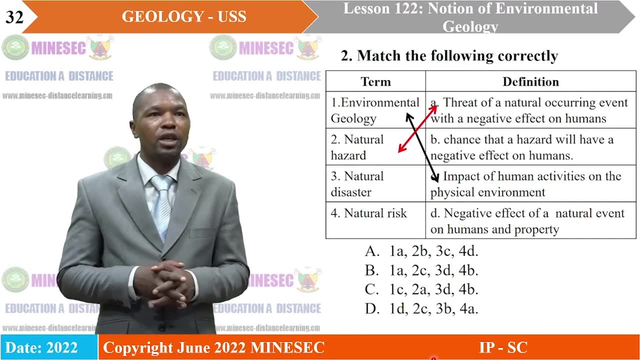 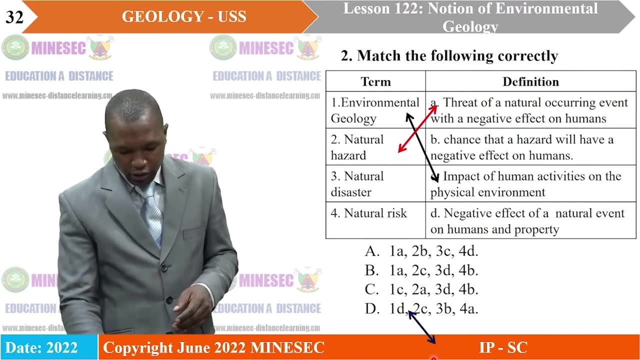 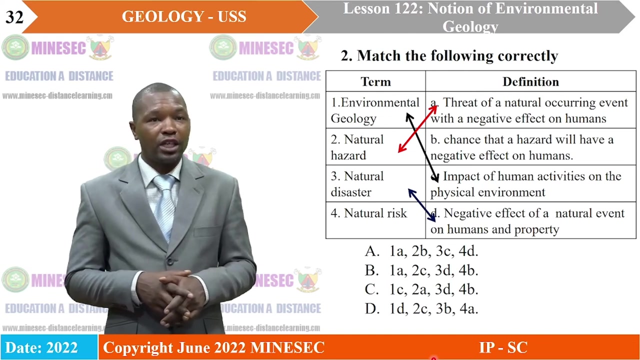 You have environmental geology relates the impact of human activities on the physical environment. Then natural hazards relates a threat of a natural occurring event with a negative effect on humans. Then a natural disaster matches negative effect of a natural event on humans and property. 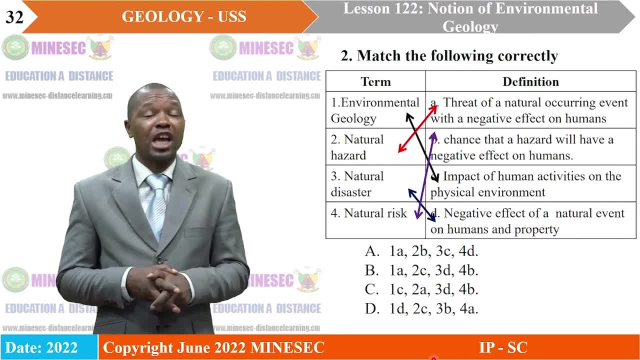 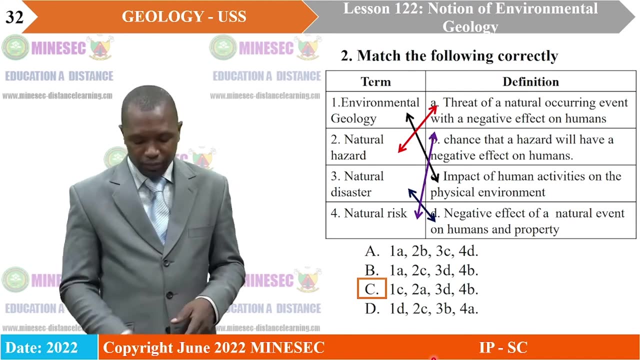 Then a natural risk matches with chance That a hazard will have a negative effect on humans. So our correct answer is C, That is, 1C, 2A, 3D and 4B. Question number three Match the following correctly: 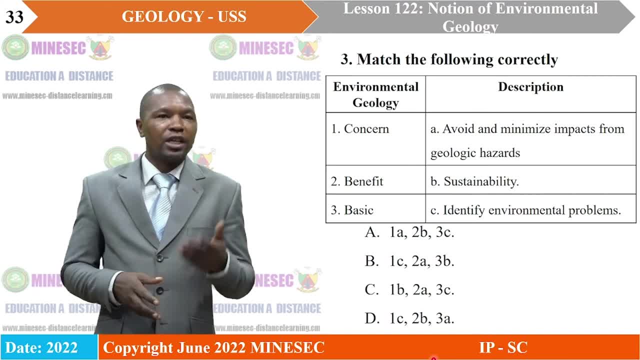 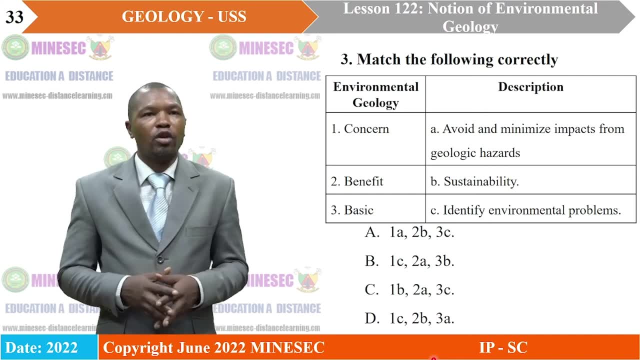 You have the environmental geology aspect, That is, the concerns of environmental geology benefits and basic principles of environmental geology, And match the following correctly: You have environmental geology benefits and basic principles of environmental geology, benefits and basic principles of environmental geology. 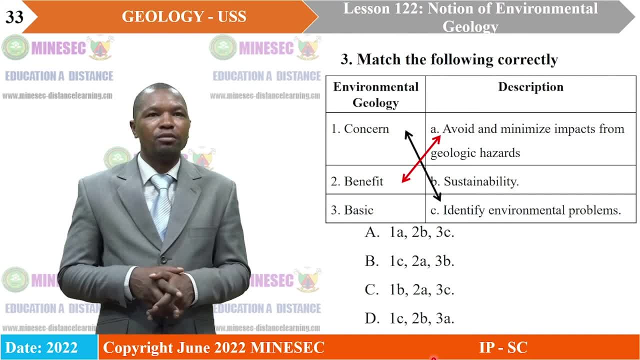 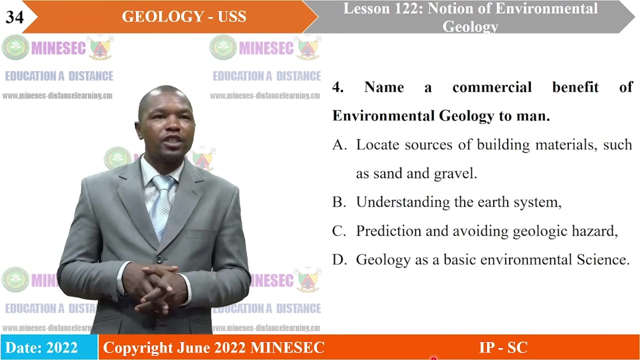 Then the benefit is to avoid and minimize impacts from geologic hazards, Then the basic principle is sustainability. So our correct answer is B, That is, 1C, 2A, 3B. Then the basic principle is sustainability. Next question: name a commercial benefit. 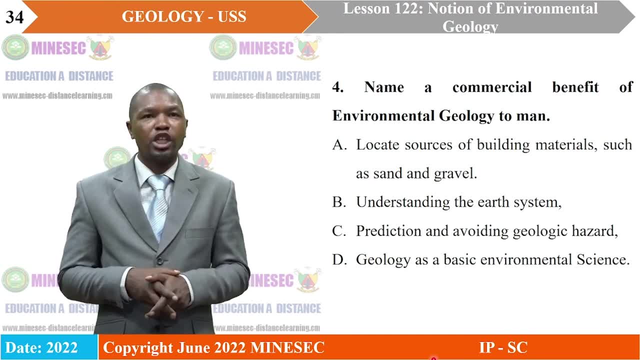 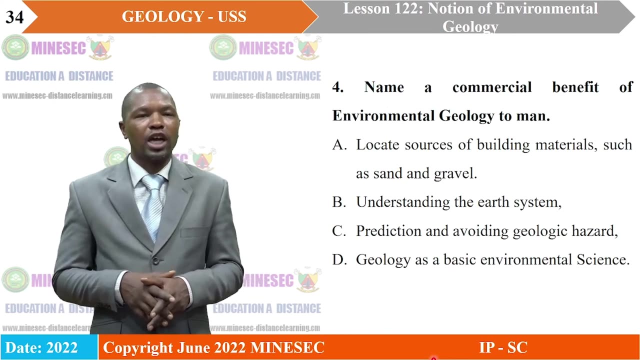 of environmental geology to man. Name a commercial benefit of environmental geology to man: A- locate sources of building material such as sand and gravel. B- understanding the earth system. C- prediction and avoiding geologic hazards. D- geology as a basic environmental science. 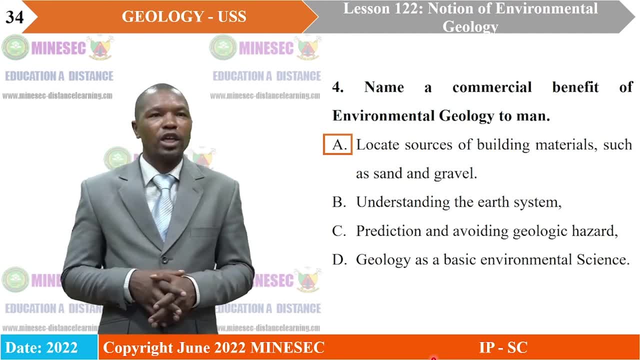 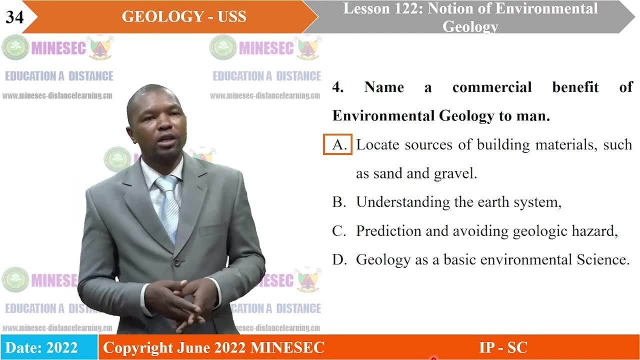 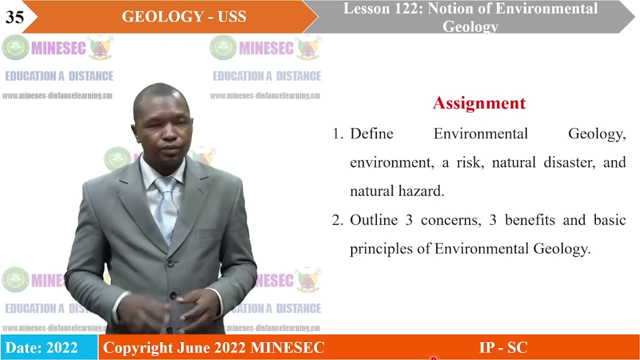 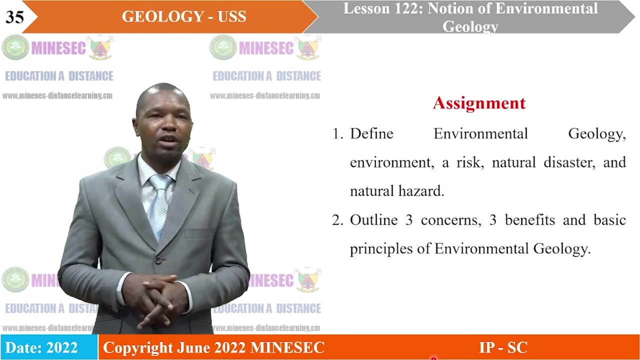 The correct answer is A locate sources of building materials such as sand and gravel. that is commercial. The rest are concerns and basic principles. As assignment, you're going to define environmental geology, the environment, a risk, natural disaster and a natural hazard. 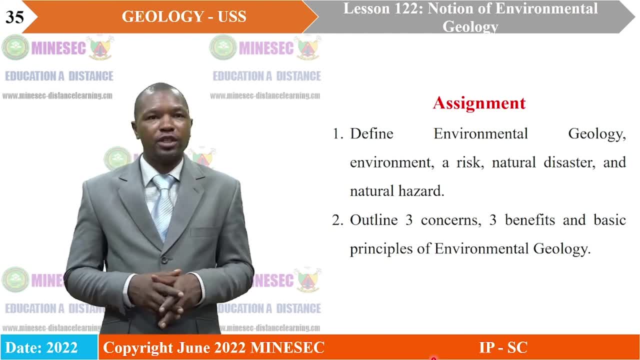 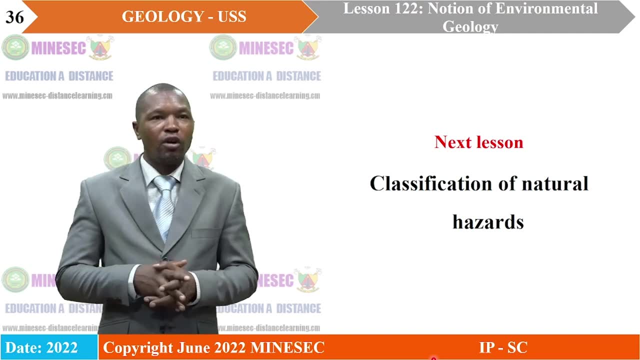 Then two outline. three concerns Three benefits and the three basic principles of environmental geology. You can also exploit more of this lesson through the use of different references, And so this way we have come to the end of our lesson on classification of natural hazards.